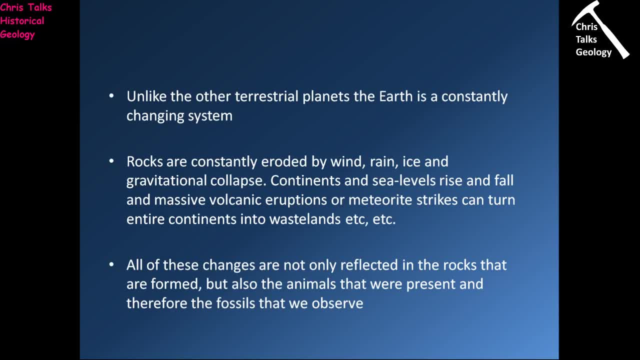 Earth is constantly being reshaped. We have continents that are moving around. sometimes they'll crash into each other, sometimes they'll rip themselves apart. We have sea levels rising and falling, we have massive volcanic eruptions and we even have the odd meteorite strike. 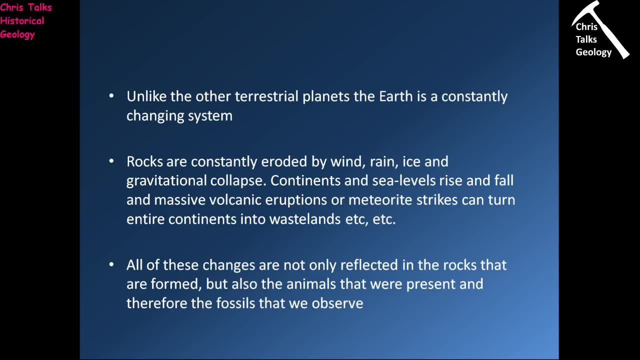 And all of these variables, you know, can produce changes in the climate, or should I say climate and the environment, on both a local, continental or even, in some cases, on a global scale. So all the changes are not only reflected in the rocks which are formed, but also in the animals. 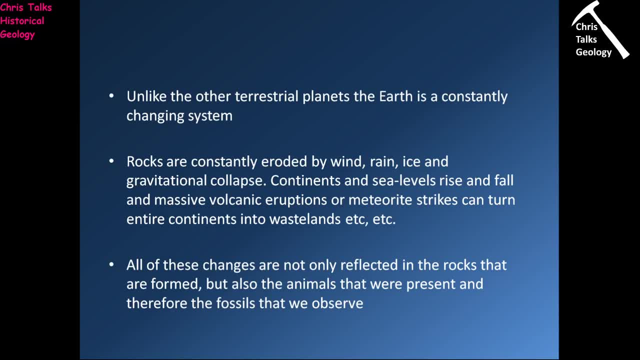 that were present and therefore the fossils we observe. So sedimentary rocks are extremely helpful to us because the sediment itself is a direct reflection of the environment, but also, on top of that, we have the additional information from the environment. So the fossils will also help us to gauge what type of environment our sediment was. 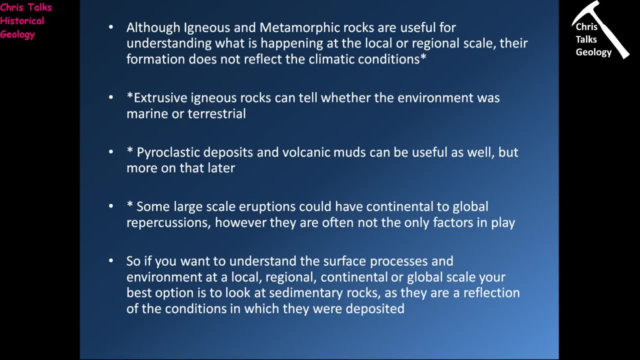 being deposited in. So igneous and metamorphic rocks are useful for understanding what's happening at a local or regional scale, especially in the subsurface. However, their formation does not reflect climatic conditions, So there are a few occasions where igneous rocks can be somewhat helpful in gauging what was going on. 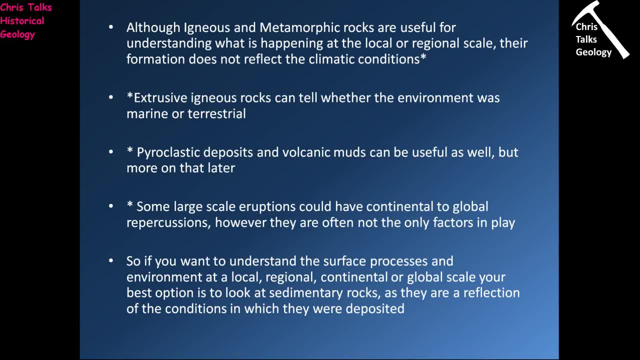 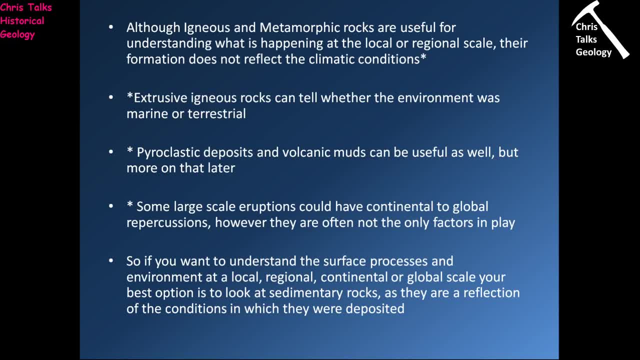 So the examples of those situations would be something like in extrusive rocks, like a lava flow, especially you know if it's a mafic lava flow like a basalt. Well, when you look at the lava flow itself, you can tell was that lava flow erupted onto the surface. 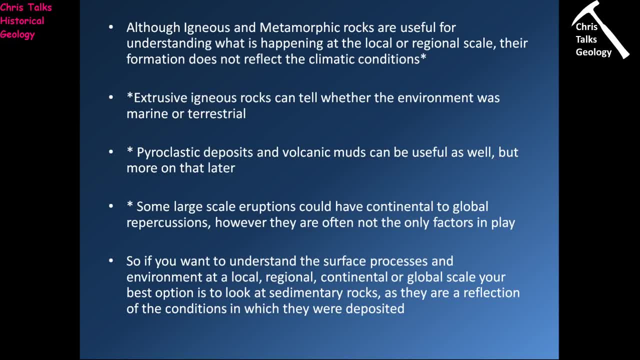 of the earth, or was that lava flow erupted onto the sea floor? So not a whole lot of information, but it does tell you. you know whether you're in a marine or continental environment. We have pyroclastic rocks. We have pyroclastic rocks. 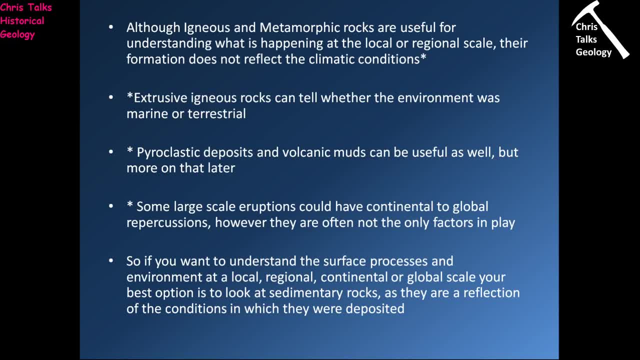 We have pyroclastic rocks, aclastic deposits and volcanic mud flows, and they can be useful as well, because sometimes, when they occur, they can actually envelop and encase plants and animals, preserving them as part of the flow, and we can also have some large-scale eruptions that can have continental to global repercussions. 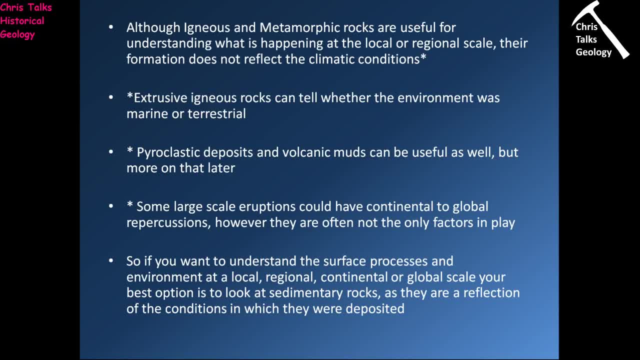 so when there's a very, very large volcanic eruption, you can actually put so much ash into the high atmosphere that some of that ash will actually reflect sunlight back into space and this can cause a noticeable decrease in global temperature. however, such an effect is typically only short-lived, you know. it'll maybe last one, maybe two years at most. so it's not. 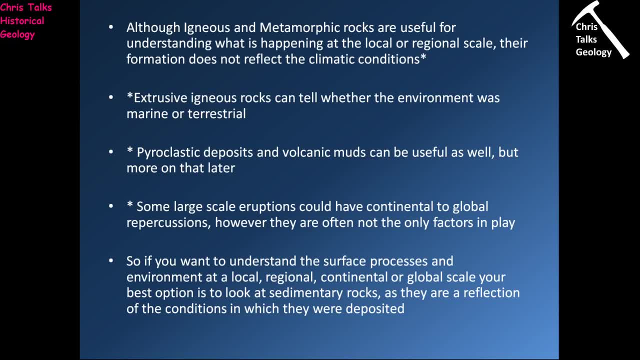 really going to have a very significant effect on global environment. so, when it really comes down to it, if you want to understand the surface processes, the environments at a local, regional, continental or global scale, your best option is to look at sedimentary rocks and, of course, the sedimentary rock is a direct reflection of the conditions in which the sediment is. 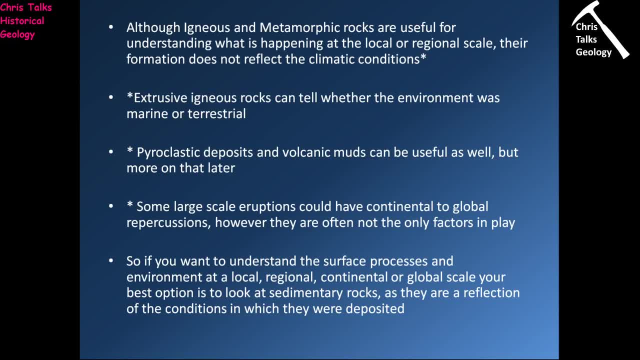 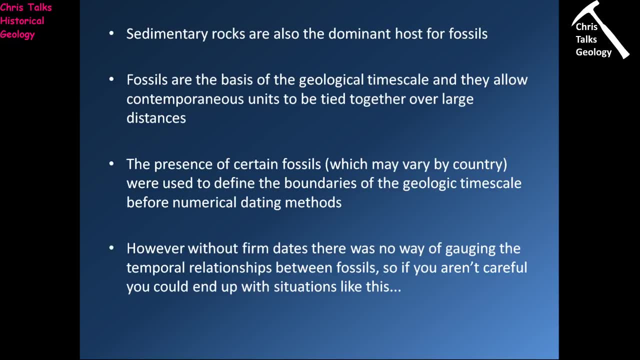 being deposited, so the sedimentary rock has indicators of the environment also. on top of that, of course, sedimentary rocks are the dominant host for fossils, and fossils are extremely useful for geologists. so fossils are, of course, the basis of the geologic timescale and they allow us to 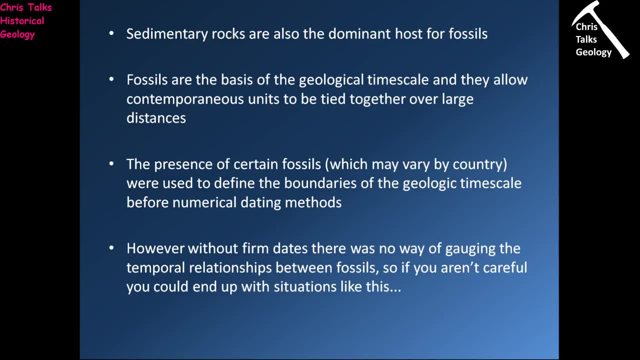 link together contemporaneous units. so we know. we've looked your geologic timescale, you know all the boundaries between the different sections of it are defined almost exclusively by the first or last appearance of certain key fossils. fossils are also helpful because they allow us to link. 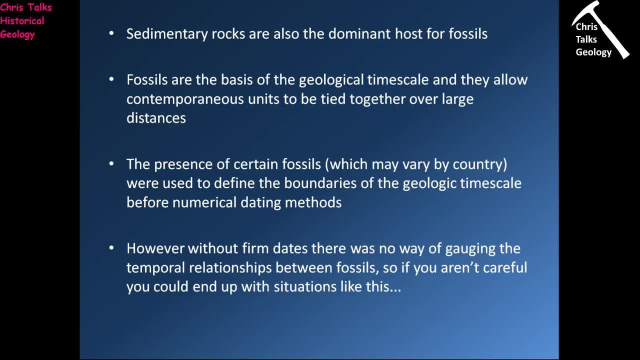 rocks together of the same age. so if i have fossil a at a location, let's say houston, texas, and i find a rock somewhere else in the world- let's say madrid, spain- and that rock also contains fossil a, well i can link those two rocks together using the fossils and i can say right. 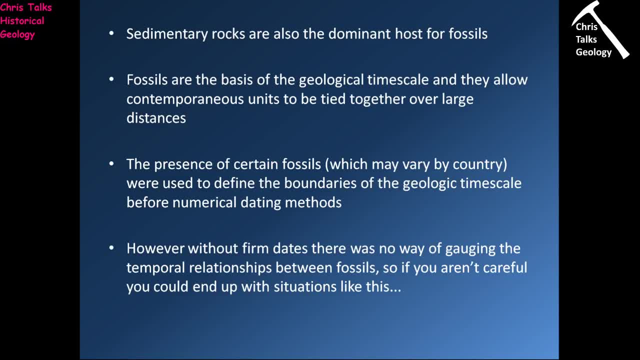 those rocks formed at the same time could have formed in completely different environments, but as long as they have the same fossil we can say: you know definitively that right, those rocks must have formed, you know, contemporaneously with one another. so we obviously have the presence of certain fossils, which will vary by country are used to. 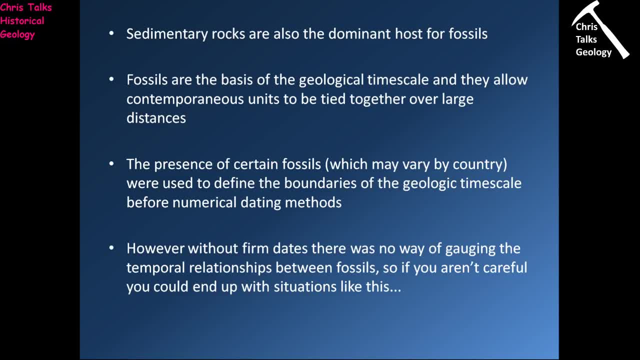 define the geologic boundaries. obviously that was before we had numerical dating methods. however, without firm dating methods, there was no way to define the geologic boundaries, there was no way of gauging the temporal relationships between fossils. so this is obviously a bit of a problem. so if you have a sequence of rocks, you might look at that. 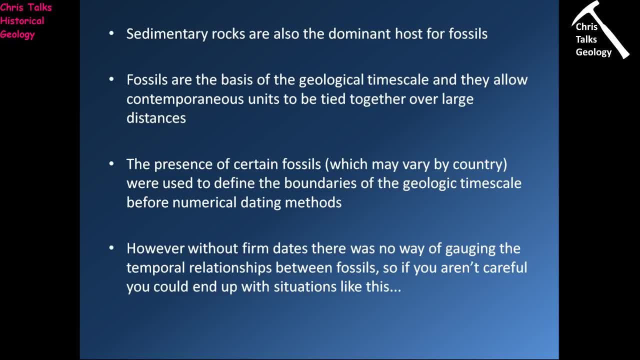 sequence of rocks and you think right. well, you know this sequence of rocks, you know it's quite thick. maybe it represents, you know, 10, 20 million years worth of accumulated sediment. in reality, it could represent 1 million years of accumulated sediment, or it could represent 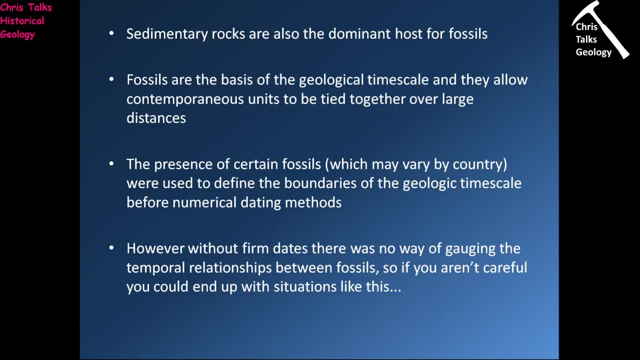 500 million years of accumulated sediment. you don't know if you can't date the rock, so you have no idea how much geologic time what you're looking at actually represents, and so that can lead to situations like this. so this is one of these classic diagrams. you 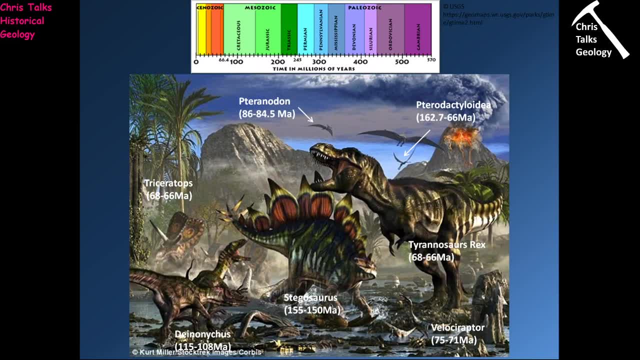 know you've seen- chances are in fact, you had a book like this when you're a child. it was a dinosaur book and in it you had these pictures where you have all these different dinosaurs all interacting and doing their thing. the problem is is that when you actually look, 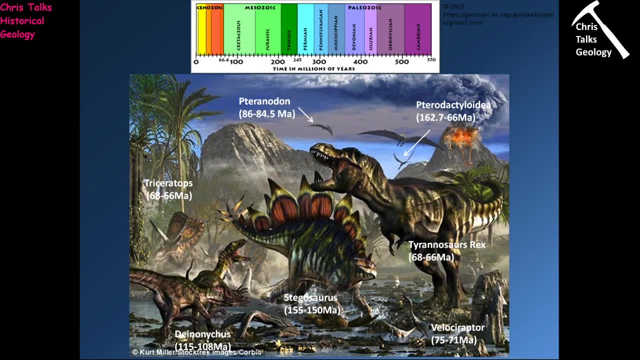 at the picture and look at the animals in it and work out when the dinosaurs actually would have been able to exist. you know, you very quickly come to the conclusion that you're very quickly come to the conclusion that they possibly couldn't have co-existed together. 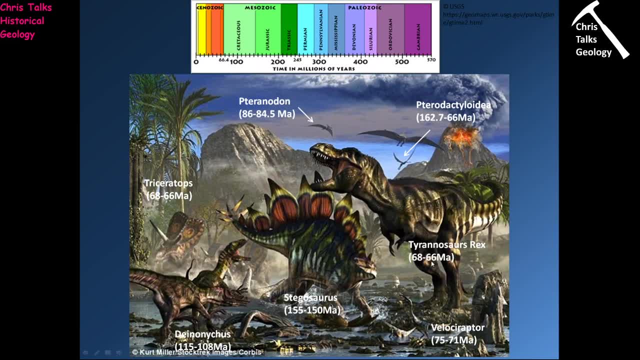 I mean, you know, Tyrannosaurus Rex was between 68 and 66 million years ago. Stegosaurus is, on the other hand, 155 to 150. they would never have occurred together, ever. but this is one of the problems if you don't understand the actual temporal relationships of the layers. 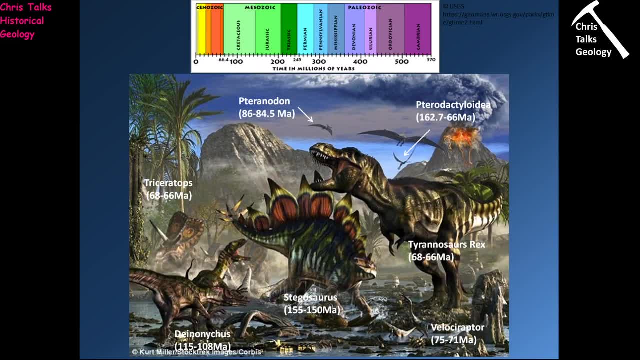 of rock, this kind of mistake can happen quite easily. so if I have a sequence of rocks and in one layer from the Jurassic I have some Stegosaurus fossils, and then the layer directly above it, I maybe have a Tyrannosaurus Rex fossil, and I have no idea what the actual ages of those layers are. well, 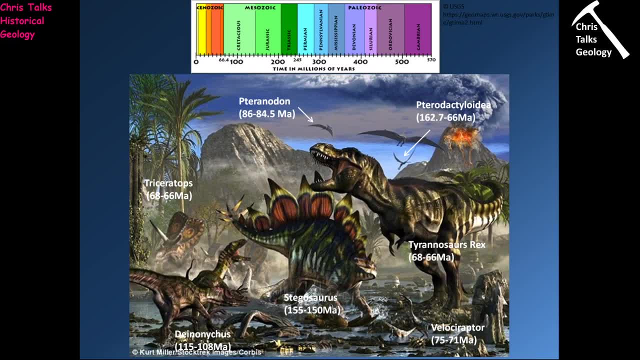 I look at one there and I say, right, well, it's a Tyrannosaurus Rex fossil directly above this Stegosaurus fossil. therefore, chances are they existed at a somewhat similar time in geologic history. I would be completely wrong, but based on a very, you know, superficial. 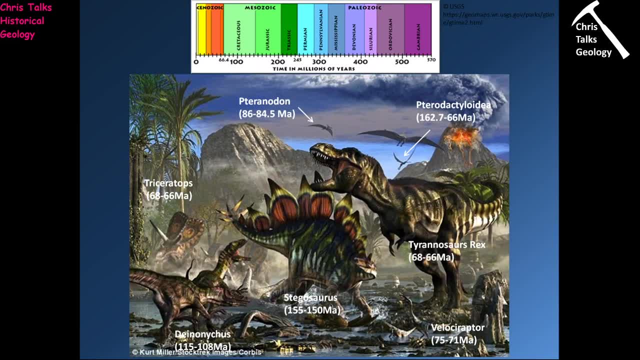 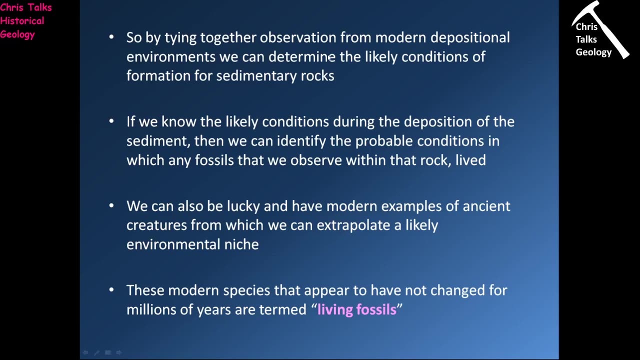 examination of the rock face. that could be the kind of conclusion you could come to, and this is one of the problems that faced early geologists: They just didn't understand exactly how much time the rocks they were looking at truly represented. So by tying together observations from modern deep situational environments, we can determine: 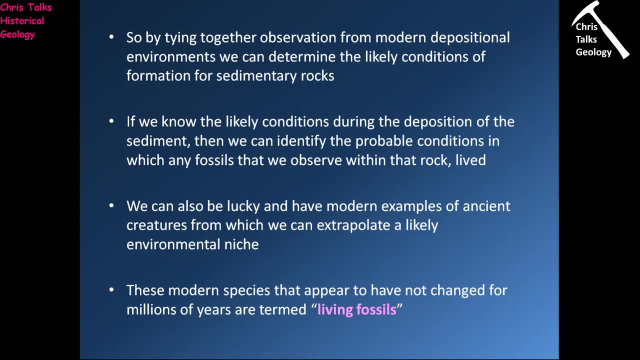 the likely conditions of formation for sedimentary rocks. So sedimentary geologists will go out to you know every deep situational environment they can think of and while they're there they'll look at the different things going on. so they'll look at the type of sediment. 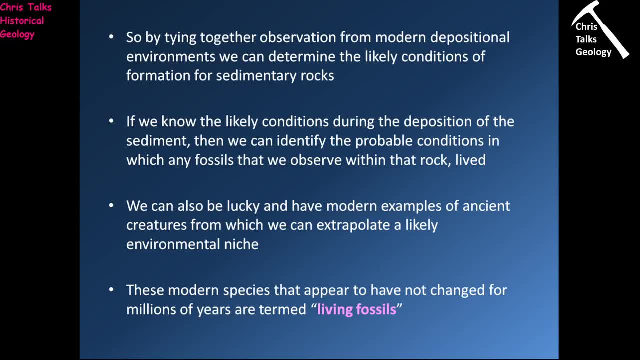 You know what's the class size, how well rounded the class, how well sorted the class, what are the class made from? then they'll look at things like textures. are there ripples, you know? are there mud cracks, you know? are there indicators of what's called a unidirectional flow? so 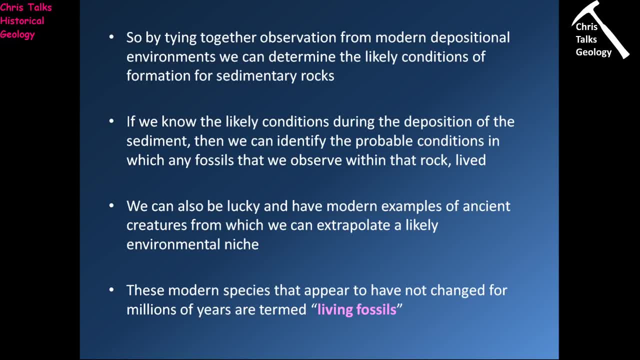 you know, materials moving in just one direction, like a river. So all this information will be gathered together and what you end up with is a set of criteria which you use to define a sediment being deposited in a certain environment. and once you have those criteria, what you can then do is you can take them and you can look for the same. 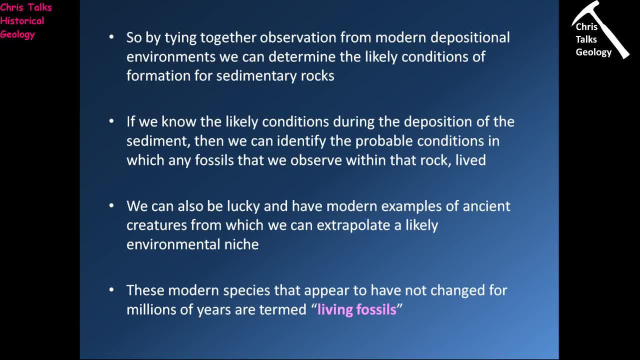 things in rocks, and so if you manage to find a rock that meets the criteria you're looking for, well then you can say, right, well, based on what I can see in that rock, that the sediment that formed that rock was deposited as part of, let's say, a delta. 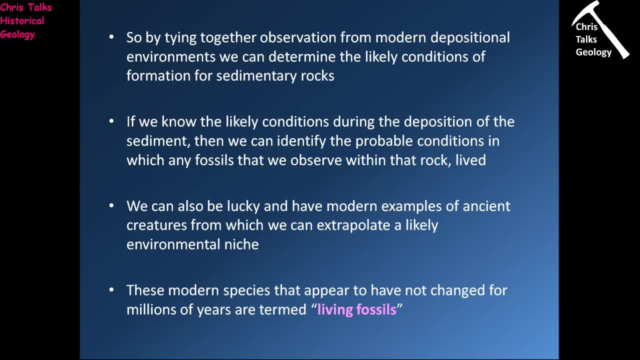 And so that's one of the great things about sedimentary rocks. the other great thing about them is, if we know the likely conditions during the deposition of the sediment, well, then we can identify The probable conditions in which any fossils that we observe within that rock would have. 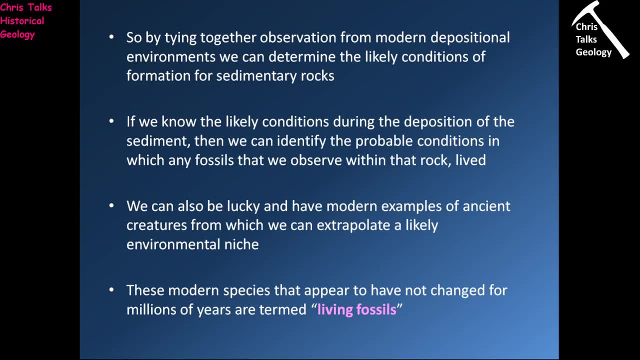 lived. so, once again, if we have our rock, which you've just discovered was part of a delta sequence, and we have fossils in it, well we can say right. well, clearly, this particular animal like to live as part of a coastal sequence associated with rivers depositing sediment. 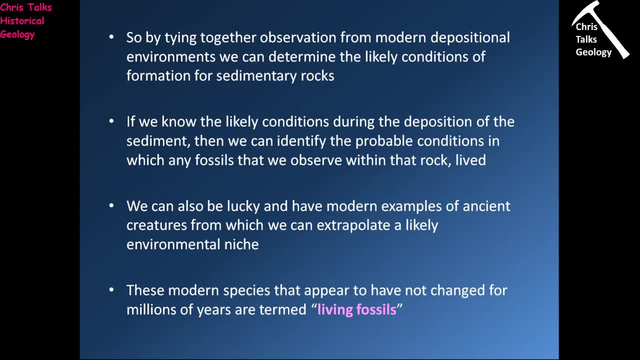 So you know, the animal probably like to live in quite shallow water, quite muddy water probably. So that's something that we can extrapolate by, you know, working out what we know where the sedimentary rock likely formed, we can then say, right, well, any fossils that we find, 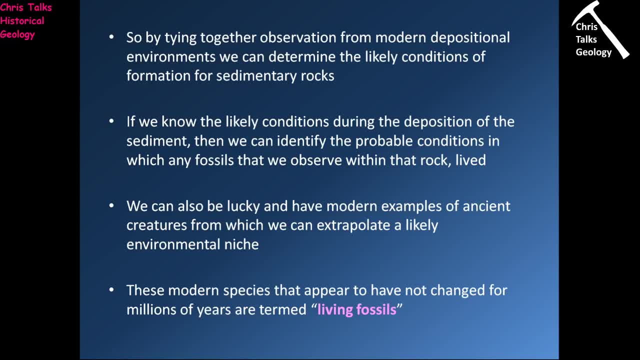 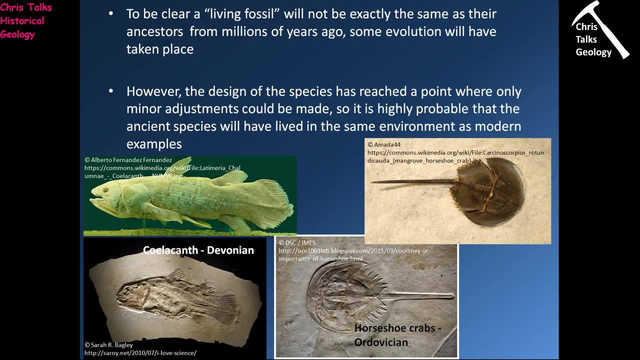 this rock would have liked to have lived in these types of environments. In some cases, we can actually get super lucky, because there are a few examples of species that appear to have not changed for millions of years, and these are termed living fossils. So, to be clear, a living fossil will not be exactly the same as that. 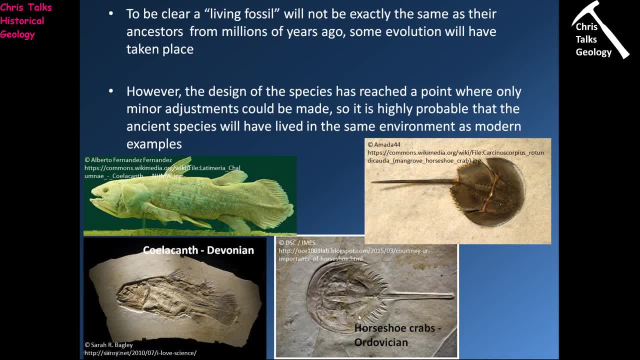 So you know, if we're looking at something like the horseshoe crab here, okay, this is a modern horseshoe crab and this is a horseshoe crab from the Ordovician, so this is about 470 million years old, And so what you can see here is you can see that look at the basic design practically. 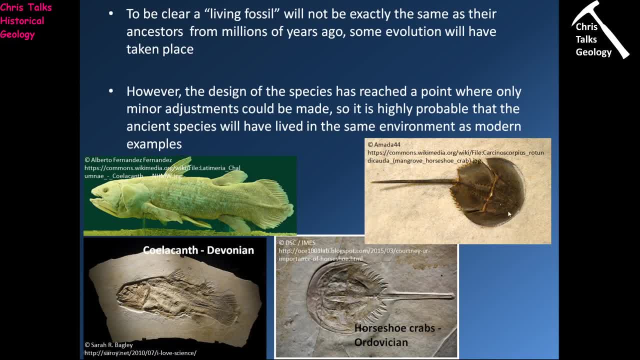 the same. So what you can do is you can extrapolate, you can say: right, well, the reason the design hasn't changed is because the horseshoe crab is so perfectly suited to its environment. So that means It's so perfectly suited. there's no push in terms of evolution to make it adapt. 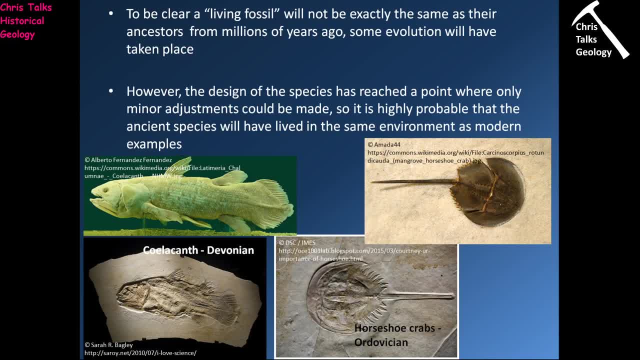 It's, it's there, it's exactly what it needs to be. And so this means that we can look at a modern horseshoe crab and we can say, right, well, chances are this modern horseshoe crab you know lived in the same environment as this ancient horseshoe. 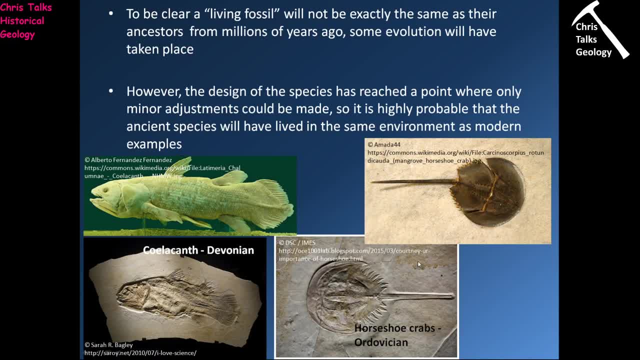 crab. So we can make that- you know- link quite easily. And here we have a type of fish called a coeliacanth. So these one, this one's from the Devonian, So it's going to be about 680 million years old. 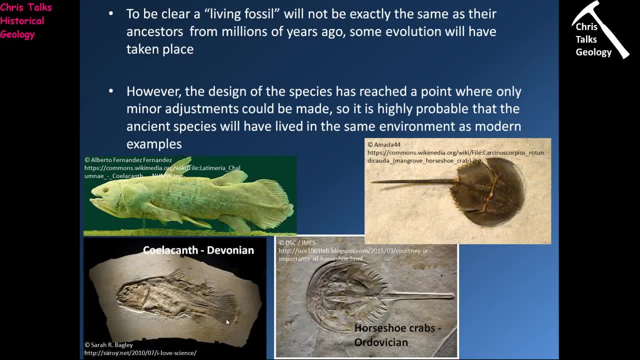 And so, once again, though, you can see the same basic design, Chances are that's because it became specialized to a certain environment. It's managed to, you know, you know, completely dominate that environment. so it hasn't died out, it's perfectly suited to it. 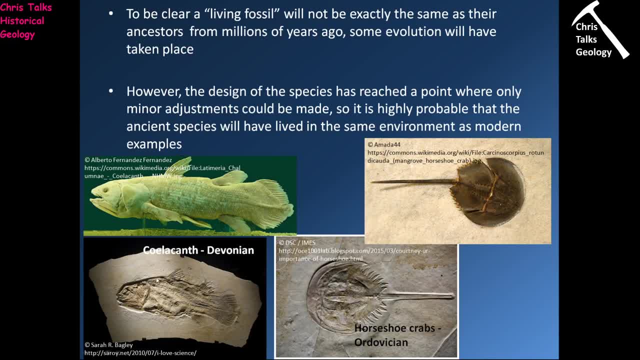 And so chances are this coeliacanth here lived in the same kind of environment as this modern example. So because the species has gone reached a point Where Very, very, very minor adjustments could be made, it's highly probable these modern examples lived in the same environment as the ancient examples. 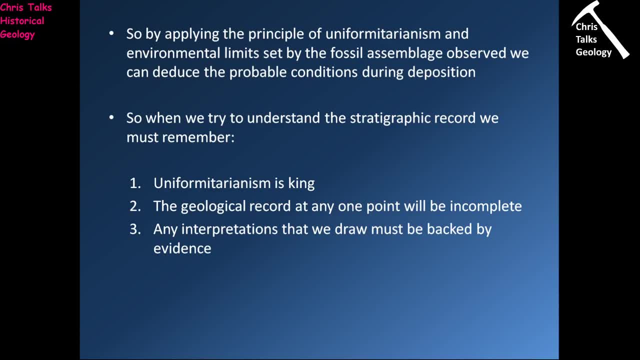 So by applying the principles uniformitarianism and environmental limit set by fossil assemblages which we observe, we can deduce the probable conditions during deposition. So when we're trying to understand the stratigraphic record, so that the rock record, we must remember three things. 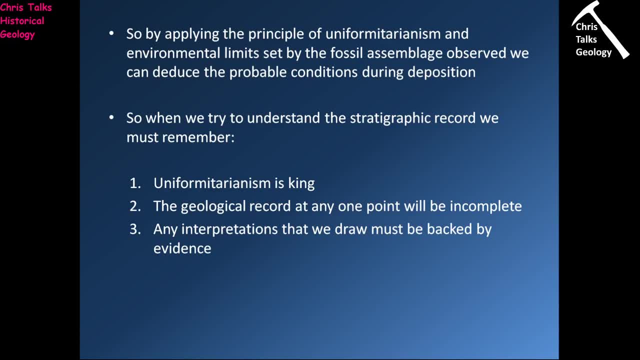 Number one: uniformitarianism is king, because that's how we work out the environment in which sedimentary rocks formed. we use modern environments and we apply what we see in those modern environments to the rock record. We also need to remember the geologic record. at any one point on the earth's surface will 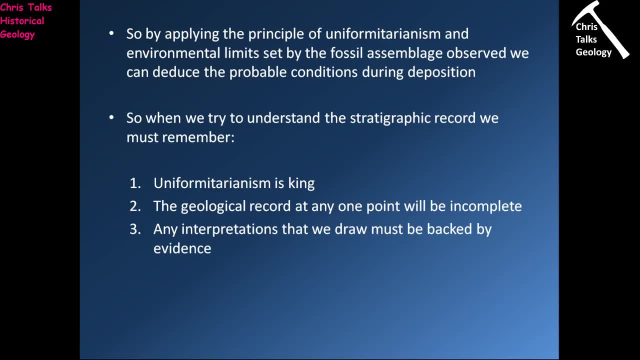 be incomplete. There is nowhere on the surface of the earth where you have the complete sequence of rocks, nowhere. And of course We need to make sure that any interpretation that we make has to be backed by evidence. we have to be able to prove one, least prove or at least firmly argue what we are proposing. 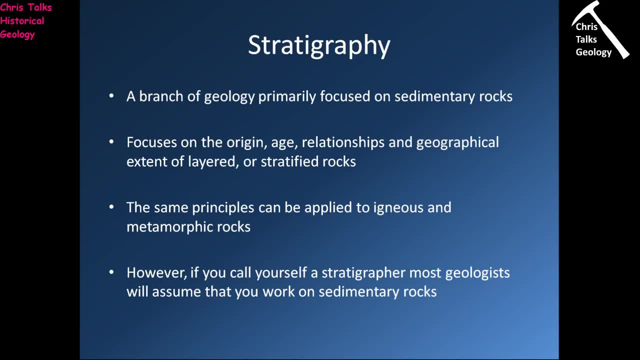 OK, so stratigraphy- a word which I have a lot of difficulty pronouncing. So it's a branch of geology primarily focused on sedimentary rocks. So it focuses on the origin of those rocks, the age of those rocks, the relationships between rocks And the geographical extent of layered or stratified rock. 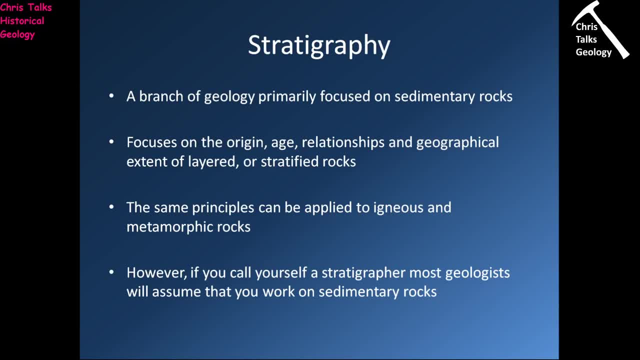 So a layered rock is considered to be a stratified rock, So the same principles can also be applied to igneous and metamorphic rock. So if you think of a sequence of lava flows, you've got one lava flow on top of another, on top of another, on top of another. 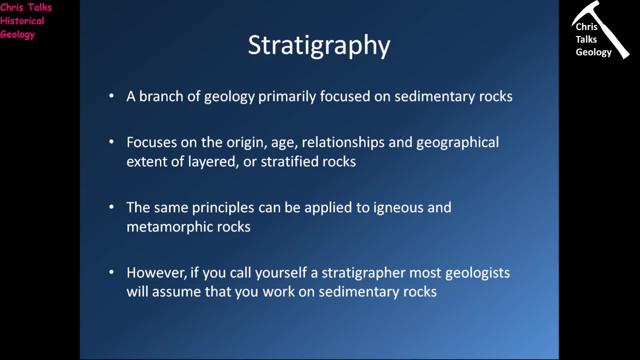 It's kind of like. you know. it looks similar to a sequence of sedimentary rock, So you can apply the same principles. However, If you actually meet a geologist And they describe themselves As sedimentary rocks, As a stratigraphy, it in all likelihood means they work with sedimentary rocks. 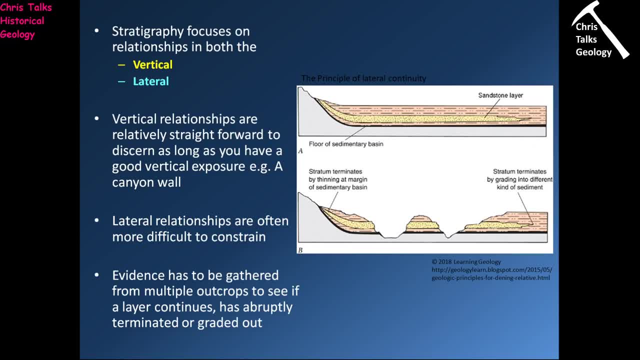 So stratigraphy is focused on relationships in both the vertical and the lateral. So vertical relationships are relatively straightforward. So as long as you have a good enough exposure, you can see what was going on. So you look at the rock in the bottom of the sequence. 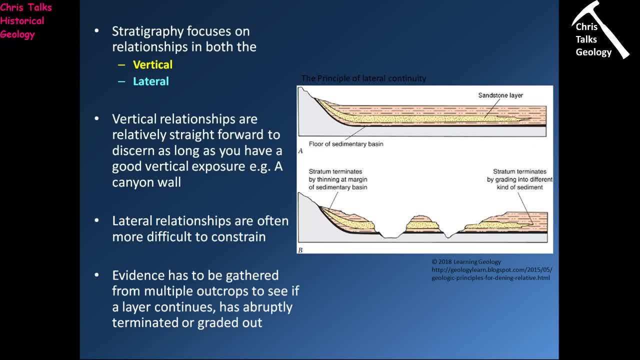 Principle of superposition says that's going to be the oldest, And then you simply work your way up the sequence, One layer of rock at a time, And you work out what you know what deposition environment each layer of sedimentary rock represents. So vertical relationships are very straightforward. 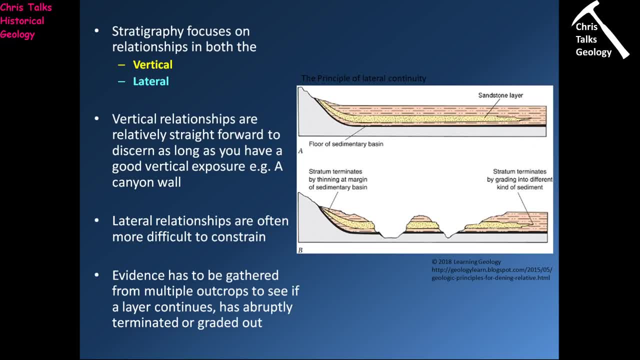 Now. lateral relationships, on the other hand, are often a little bit more difficult. So in order to work out what's happening to a layer of rock- And let's use our sandstone here as an example- We would need to travel to multiple locations. 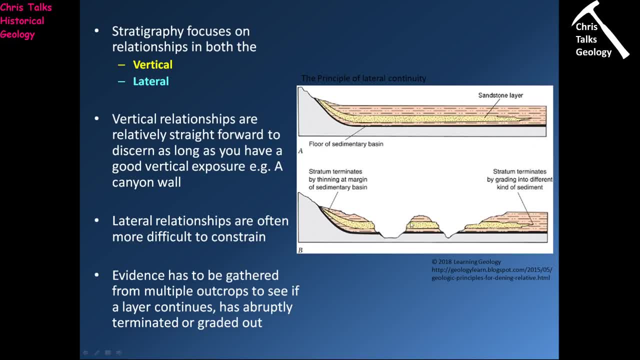 So if we're just looking at the vertical relationship, We could just stand here At the bottom of this cliff, Look at the sequence there And we could work out. you know what was going on in the vertical. However, horizontally, we would need to go to multiple locations and track the same layer. 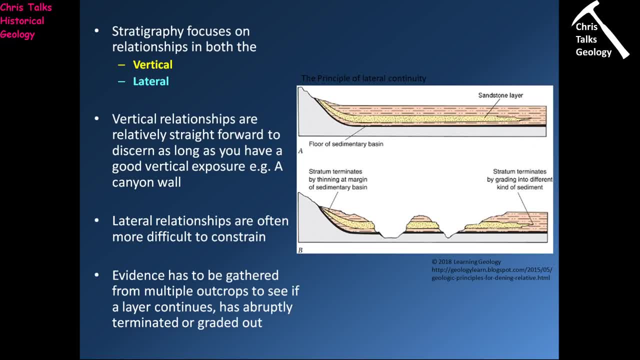 of rock And, as we know from the principle of lateral continuity, eventually the layer of rock will pinch out and disappear or it will terminate against some kind of basin margin. So this is why lateral relationships are quite difficult, because you have to go to multiple locations. 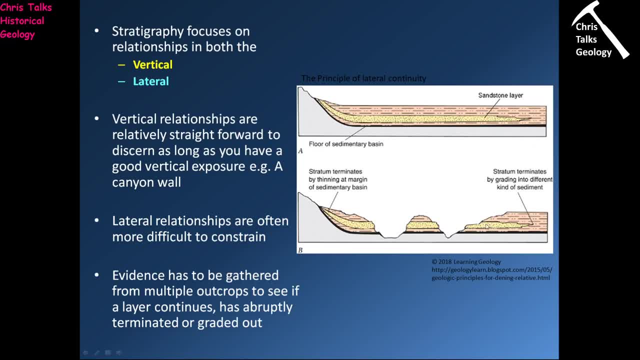 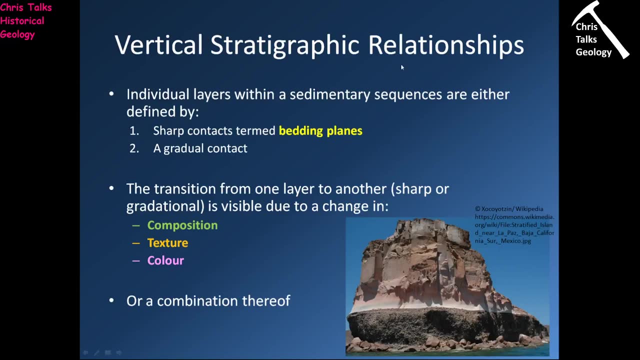 And in some cases You know the locations you would like to go to just aren't there. they've been completely eroded away, so the layer of rock will just completely disappear. So this is a bit of a problem for geologists. So let's think, let's start by looking at the vertical stratigraphic relationships. 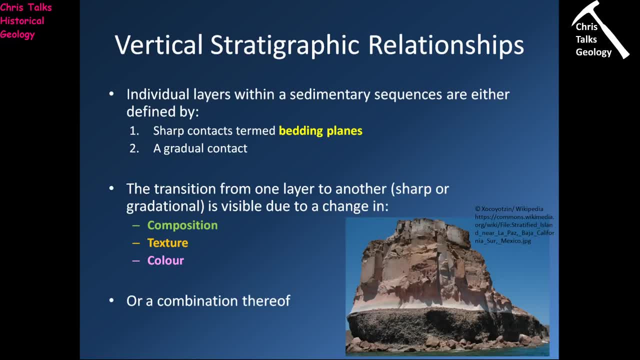 So individual layers within a sedimentary sequence are either defined by sharp contacts, which we call bedding planes, or gradational contacts. So if we look at this picture down here, we can see we have two distinct layers of rock. We have this darker, rubbly looking layer which is a conglomerate. 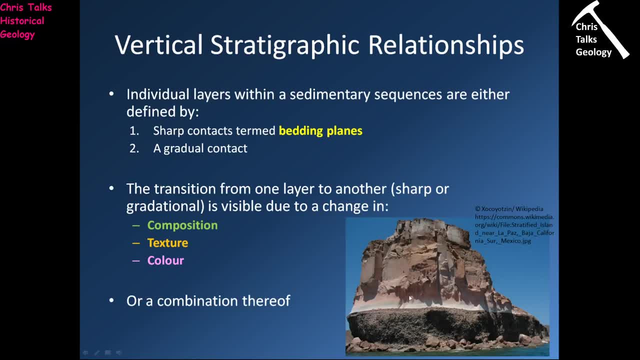 And then above it we have this blocky kind of pinkish white layer which is a limestone, And you can see between them we have this nice sharp boundary. That's our bedding plane, So when you are looking at a rock face You can pick out the individual layers. 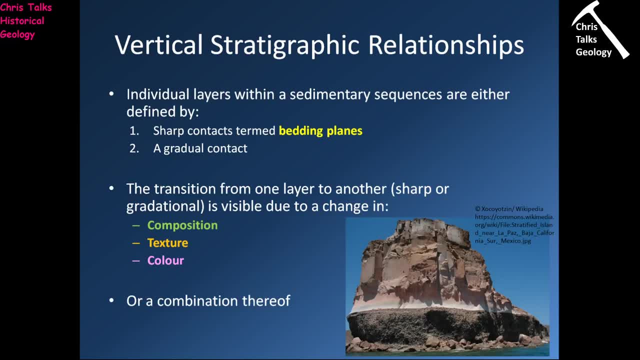 Quite easily, And that's because as you go from one layer of rock to another, there's going to be some kind of change and you can see those changes. So the changes that we see could be something like composition. so if we look at this picture, 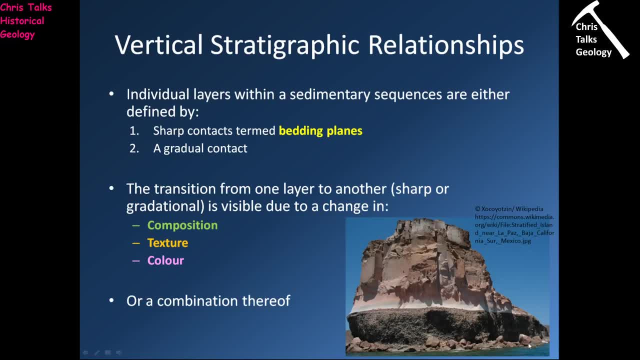 down here. Well, what can we see? Well, we can see. down here we have a rock that's made from quite large chunks of rock. In contrast, this rock up here is made from calcium carbonate. so we have a difference in the rock chemistry. We also have a difference in the texture. 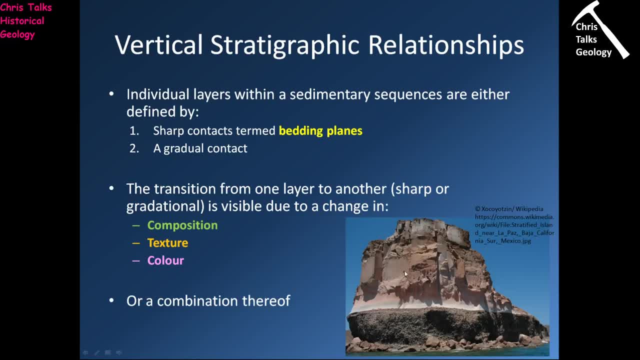 We can see this is a very rubbly texture. This is a very massive and uniform looking texture And obviously we have differences in the colour as well. This one is kind of black brown and this one is kind of pinkish white. So you know, just by looking at the picture we can see here, we can quite easily distinguish. 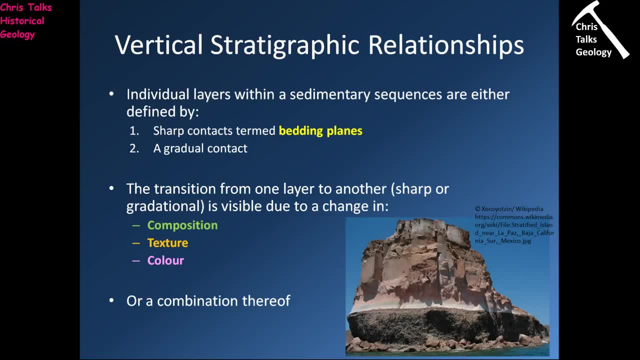 between the two layers. We don't even realise we're doing it when you know. if you look at it just for a second, you won't realise what criteria we're using to distinguish between the layers. All you know is that you can distinguish between them very easily. 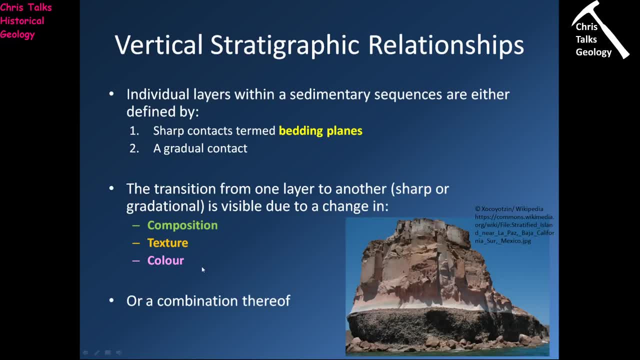 And it's because we're looking at a rock, It's because one or more of those variables will be changing and that allows you to see the change. So when we're looking at sequences of rocks, it's variations in these three factors which will make the different layers look different. 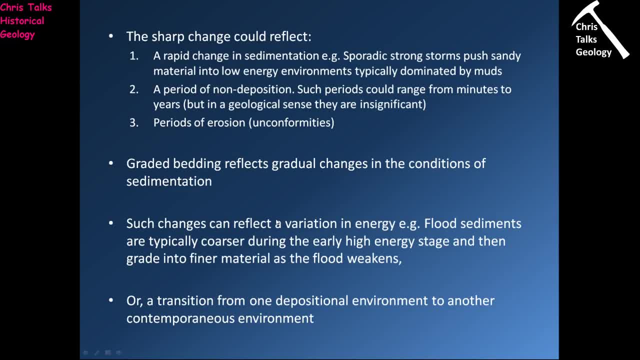 So we can discern them from one another. So when we have these sharp boundaries, it can reflect a few things. Number one: it could reflect a rapid change in sedimentation. So, for instance, if we have an environment where you know, let's say, we're off the coast. 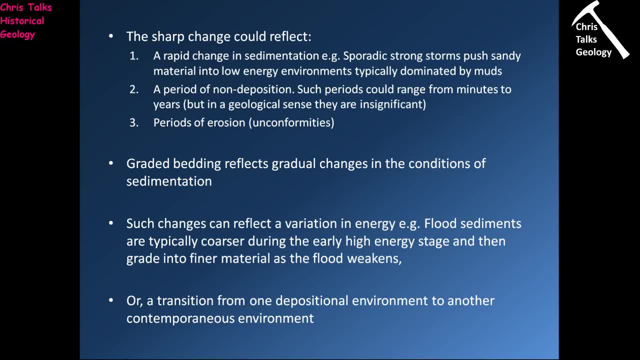 we're under water and but the environment is quite stable. well, that's an environment where you know it's quite low energy. we might have lots of muds being deposited, So we might be in a marine mud dominated environment. Now then, every once in a while, what might happen is there might be a big storm come. 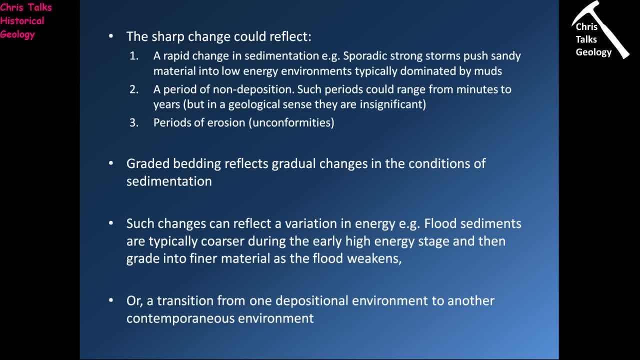 in, And that big storm will churn up the water, and it might cause some of the more sandy sediment from closer to the coast to slide down the continent, The continental shelf, And so what will happen is, all of a sudden, our muddy environment will suddenly have a 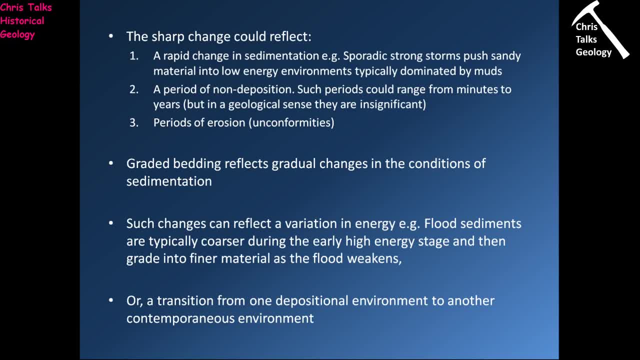 layer of sandy material dumped into it. So there was a very sudden change in sedimentation. We went from a nice peaceful, muddy environment to a, you know, a high energy environment into which this sandy material is being dumped And obviously that's going to lead to a nice sharp boundary between the two layers of sediment. 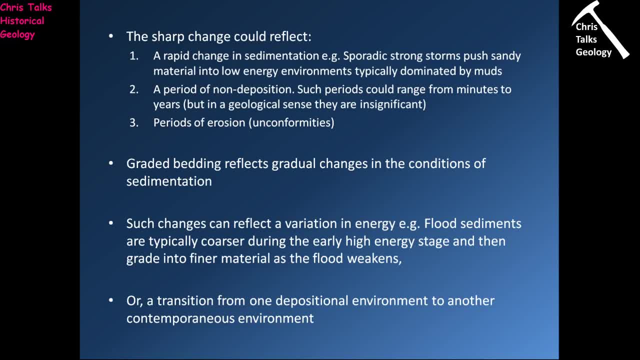 A sharp change could also represent a period of non-deep position. So if you have a situation where you're in the middle of the ocean and you've got a lot of sediment in the middle of the ocean, For instance, if we just go back to the previous picture, let's say, for a period of time we 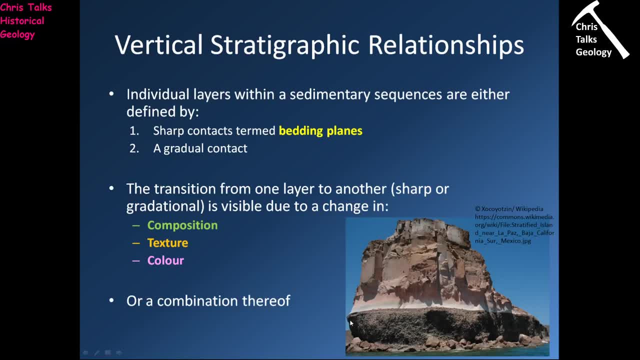 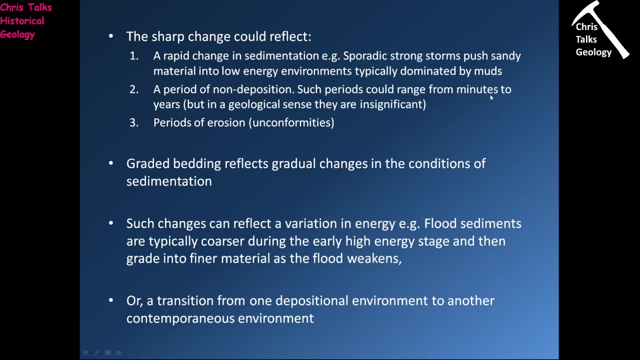 have this conglomerate forming, and then sedimentation stops for a while. Nothing's really getting eroded, nothing's being deposited, so everything just pauses for a little bit, and then this layer of sediment gets deposited over the top. Now, these periods of non-deep position could last simply from minutes through to years. 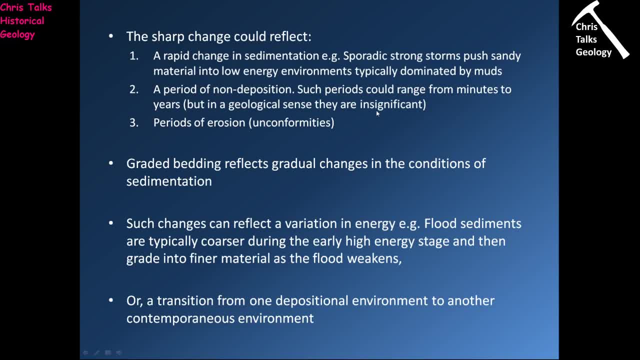 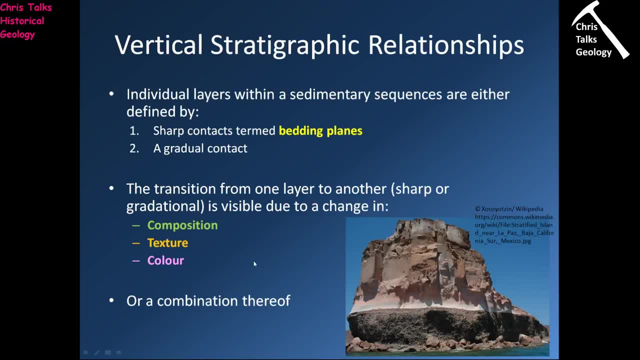 but from a geologic point of view they're insignificant. And then of course we have periods of erosion, Which of course produces unconformities. So in that case, if we just go back to this previous picture, in the case of an unconformity, 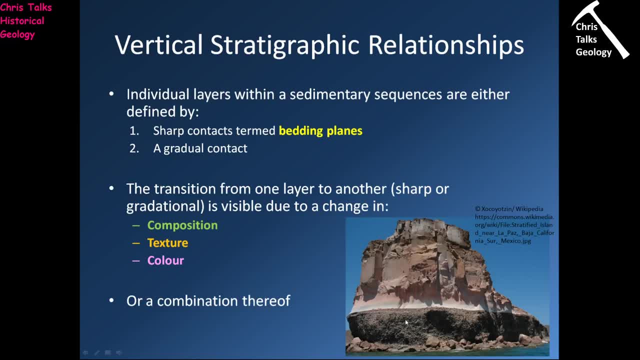 there could have been a whole sequence of rocks here, So there could have been a conglomerate, then a sandstone, then a mudstone, then a limestone. but all that stuff above the conglomerate here got eroded away. so it's gone, it's lost. 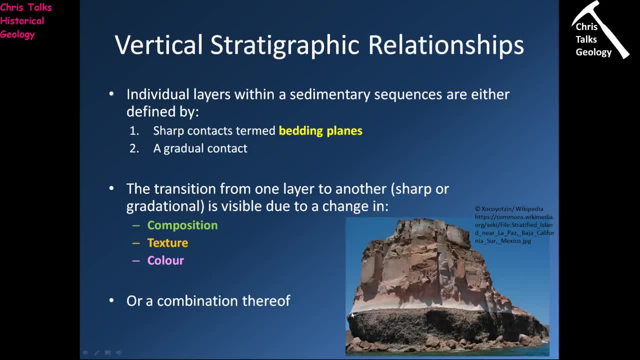 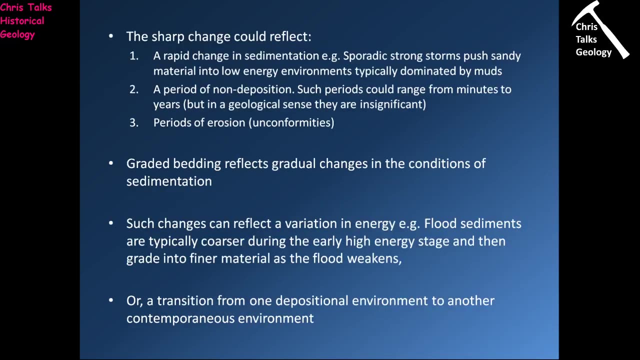 And then this limestone gets deposited over the top, And so this contact here would represent the unconformity and of course, represent lost rock And therefore lost time. But once again you would end up with a nice sharp contact. So, in terms of the other option, which is graded bedding, 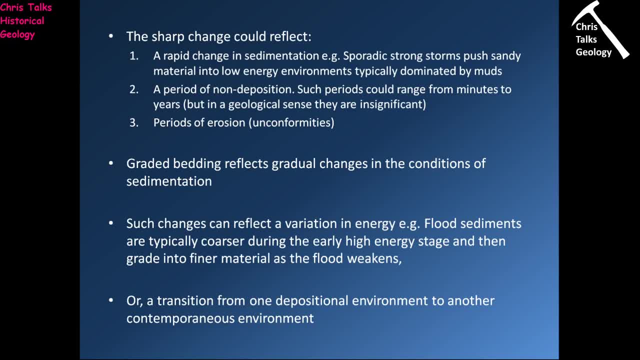 Graded bedding will reflect a gradual change in the conditions of sedimentation, So such changes could reflect a variation in energy. So think of a river flooding. Well, when the river floods, the water comes out of the river and it leaves the river with lots of energy. 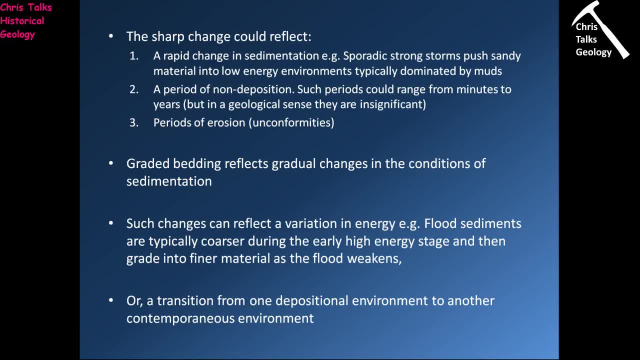 So it's carrying a lot of sediment with it. the water is quite energetic Now because it has lots of energy. that means it can move quite a large range of class sizes. It can move small clasts and it can move medium sized clasts. 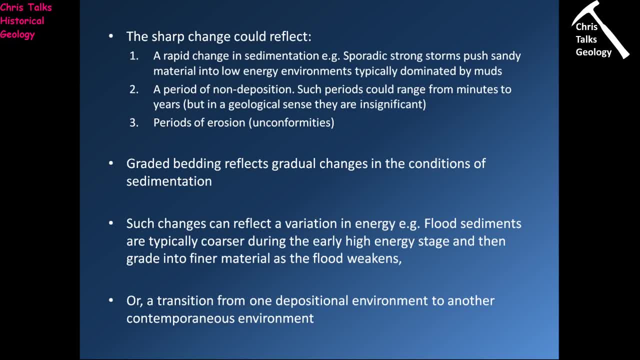 The problem is: as soon as the water starts leaving the river channel, all of a sudden it begins to slow down quite quickly. And as the water begins to slow down, first of all it has to dump the large clasts, and then, as the water gets slower, 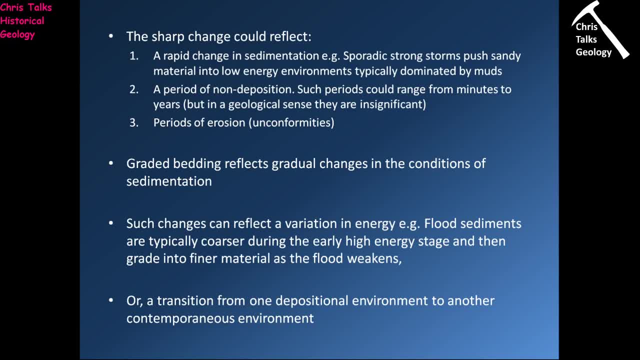 It will then dump the next size of clasts and then steadily over time, as the water gets lower and lower energy, finer and finer material will be deposited. So you know, when a river floods you might get a sequence that goes medium sand, fine sand, very fine sand, silt clay. 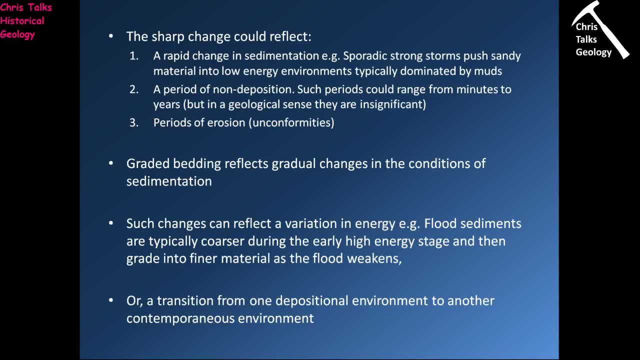 So the medium coarse sands at the bottom and the clays at the top, and that's just the result of the energy of the systems steadily changing, going from a high energy initially to a low energy at the end. We also get gradational contacts when we transition from one deep situational environment to another. 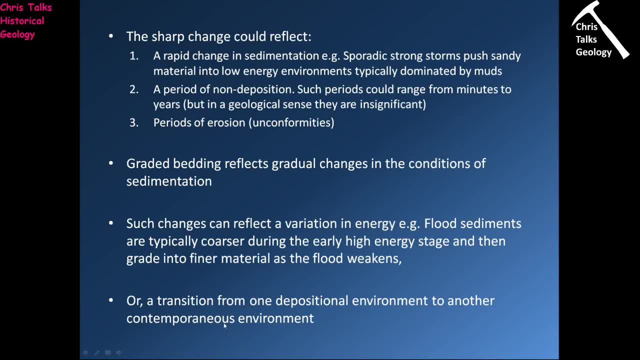 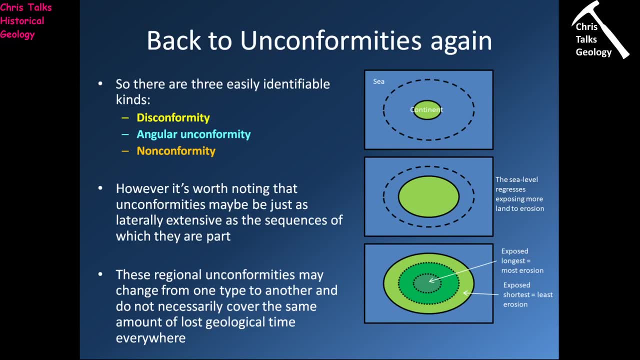 if they are contemporaneous with one another, So if these two different environments are operating at the same time. Ok, so let's think of unconformities. So, if you remember, there are actually 4 types of unconformity: Disconformity, angular unconformity, nonconformity and paraconformity. 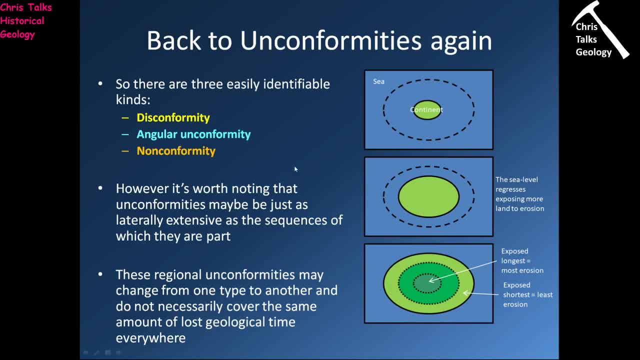 Now, paraconformities are a bit of a paradox, a bit of a pain to identify. so most of the time when we talk about unconformities, we're only really talking about the first three: disconformity, angular unconformity and non-conformity. 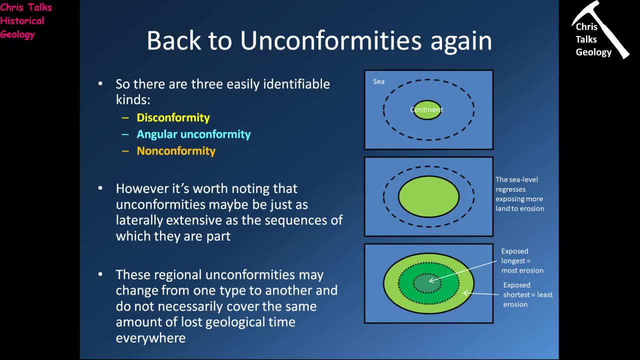 so when you're standing in front of a cliff and you can see that you have one layer of rock and maybe let's say this first layer of rock is 200 million years old, then the layer of rock above it, you can date that and it's 150 million years. well, that means the contact between those two layers. 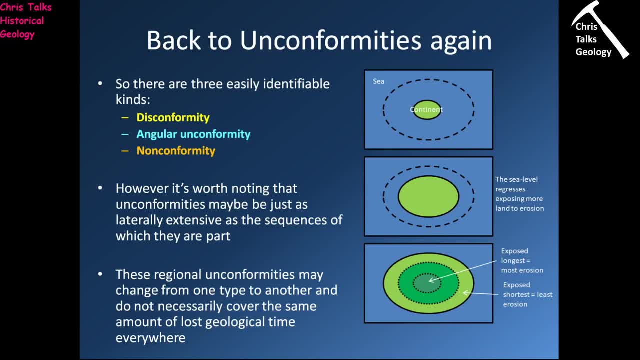 of rock has 50 million years of lost material. one layer was 200, the next layer was 150. therefore, there's a 50 million year block of time missing. so that's our unconformity. now, that is perfect when you are just looking at one location. however, stratigraphy says we don't just look. 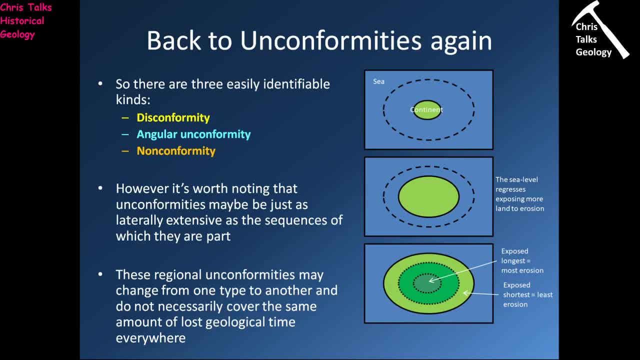 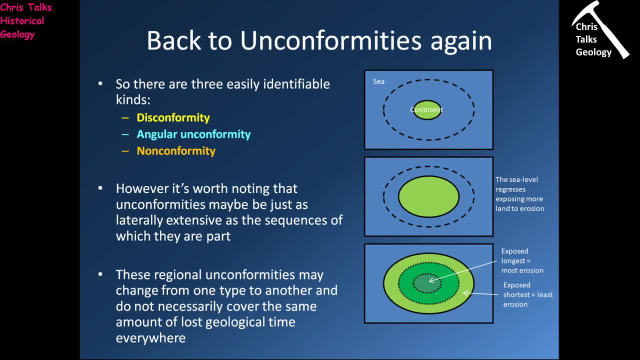 can cover entire continents. So there are some unconformities in North America that will literally go all the way from the west coast across to the east coast. they're huge. The other thing about unconformities is that an unconformity does not represent the same. 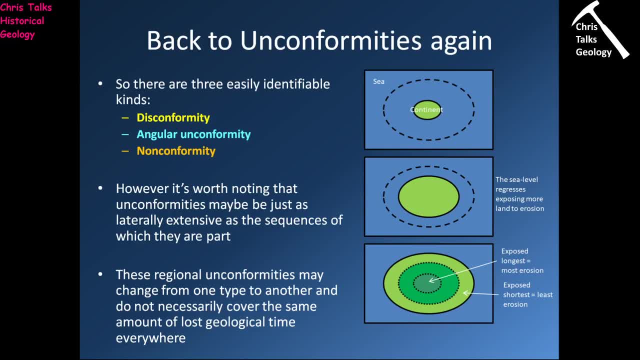 amount of lost time at every location. So over here on the right, we have some wonderful diagrams produced by yours truly, and we can see here we go. so here we have ourselves, a little continent, and it's surrounded by the ocean, and this dash line here represents 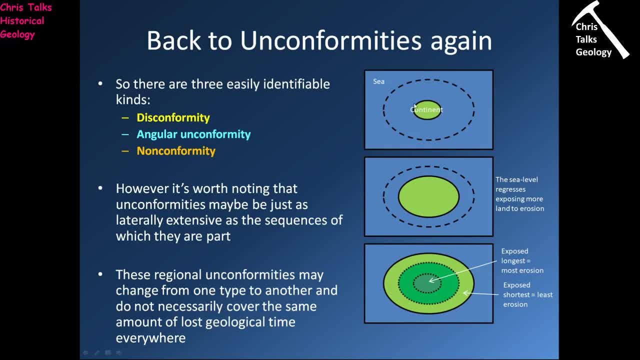 the edge of the continent, which is under water. so this green area is the bit that's exposed. Well, as it's exposed, that's the area that's undergoing erosion. Then, steadily over time, the sea level drops and so more new land is exposed. so this area is now undergoing. 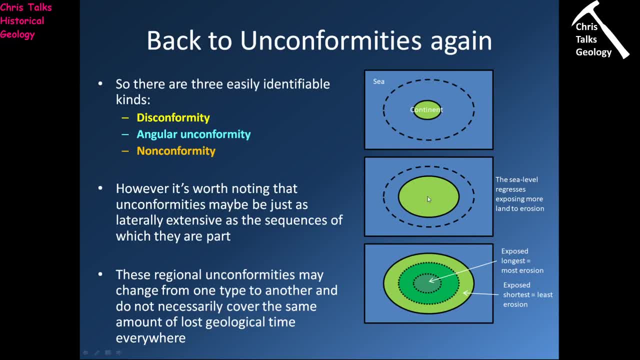 erosion. but the bit in the middle that was exposed first, well, that's undergone more so. it would have lost more rock, and then, over time, the sea level retreats until the continent is completely exposed, and by this point we'll have an unconformity running from one side. 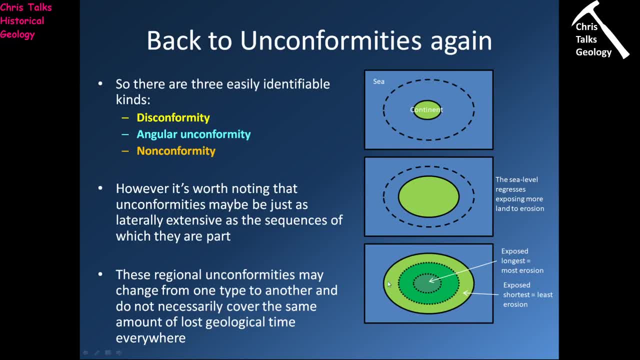 of the continent to the other, Because everything is exposed, it's being eroded, and so we're losing a rock, So we're forming our unconformity. However, the unconformity does not represent the same amount of lost time at every location. So in this area, in the centre, here, which was exposed first, we're 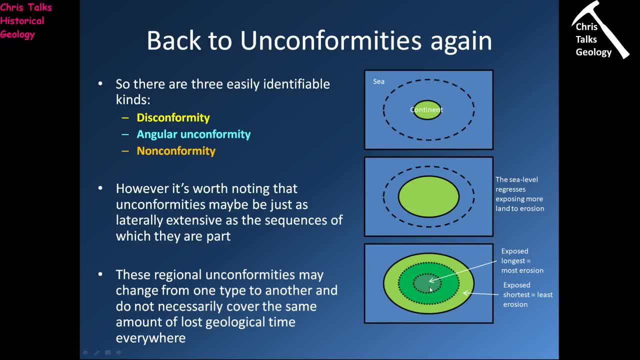 going to have an unconformity which represents a significant amount of lost time, because lots of rock has been eroded. In contrast, the rocks out here, well, they will have suffered and, as such, you will have lost less material, and so the unconformity out here will represent. 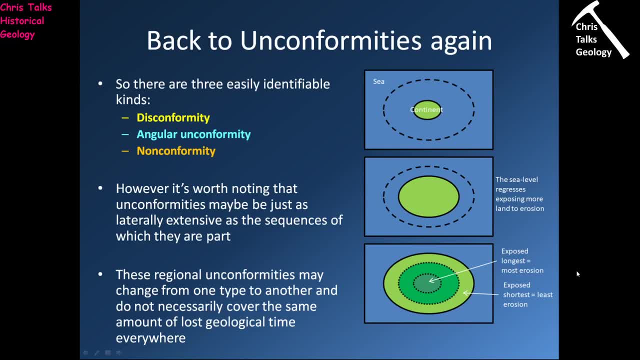 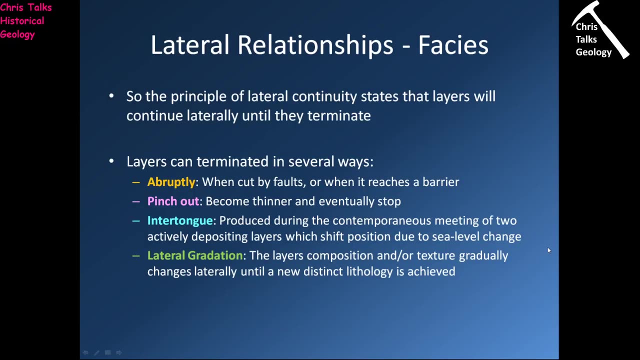 less lost time, And so we need to remember this- that when we're talking about stratigraphy, we're not just thinking in the vertical, we're also thinking in the horizontal as well. This applies to unconformities just as much as it does to layers of sedimentary rock. 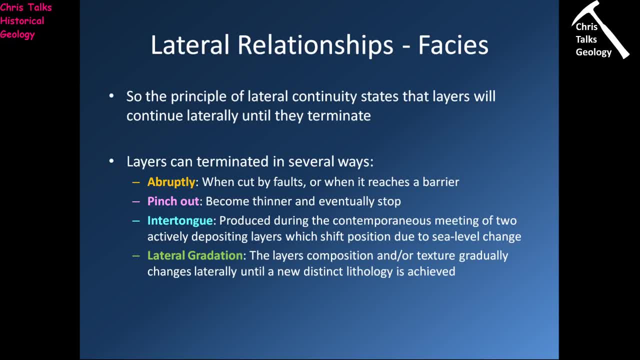 So we need to think about things which we call fascii or sedimentary fascii. So we're going to think about how sedimentary rocks will change laterally. So a fascii is simply an environment which will lead to the deposition of a distinct sediment which will form a distinct 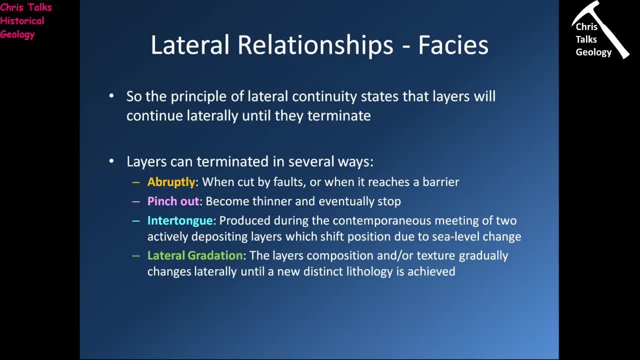 sedimentary rock. So, for instance, if you want to think of different fascii, so let's think of a coastal fascii, so let's think of a sandy beach fascii. Well, in that environment you have a beach environment. it's moderate to high energy. there's lots of sandy material. 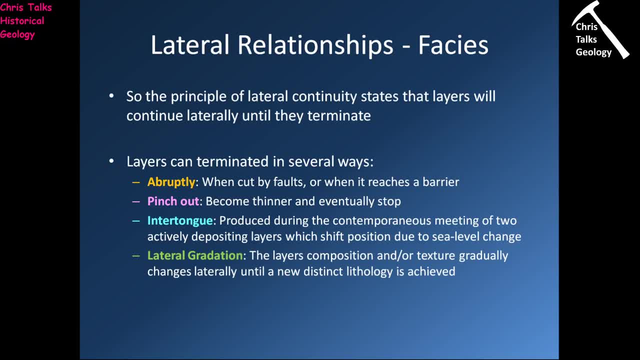 there, And so we know that environment is going to be a sand dominated environment. we're going to see ripples, we're going to see fossils, all that kind of stuff in this environment. So we can look at that package of rock and we can say, yes, this package of rock formed 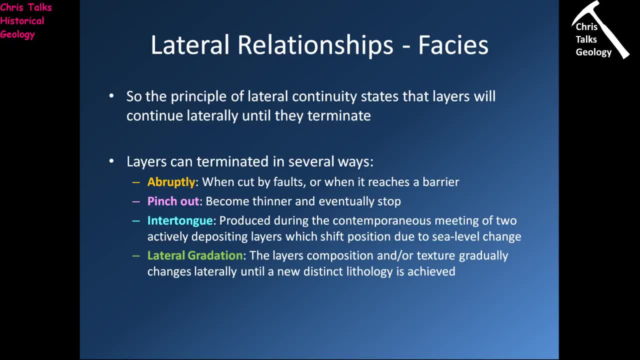 in a coastal beach environment. Now then, as we move into deeper water, so we're going down the continental shelf- eventually- the water will steadily become less and less energetic, so we'll transition from a higher energy sand rich environment closer to the continental shelf. 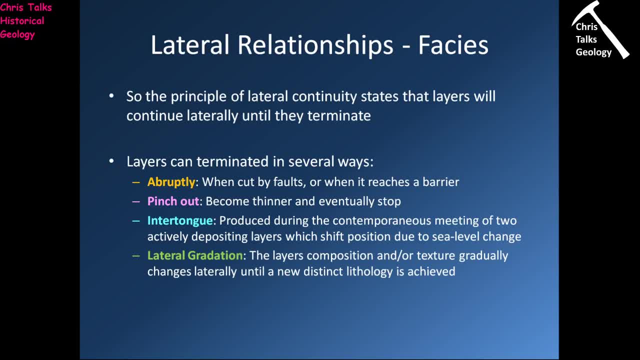 And then, as we move through the salt water, we'll go a little bit closer to the coast and we'll move into a lower energy mud rich environment further out. Now, obviously, now we have a completely different type of environment which is going to produce a completely different sediment. The beach environment produced a sandy sediment because 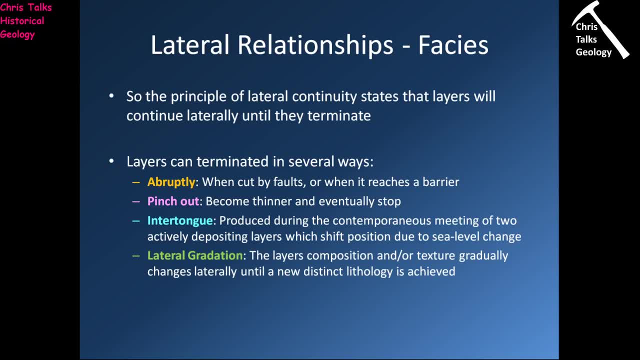 it was moderately energetic. The low energy environment, on the other hand, is going to have a mud dominated sediment, And so simply by looking at these different sediments, we can tell that we've transitioned from one environment to another. We've moved from the moderate energy environment to the low energy environment. 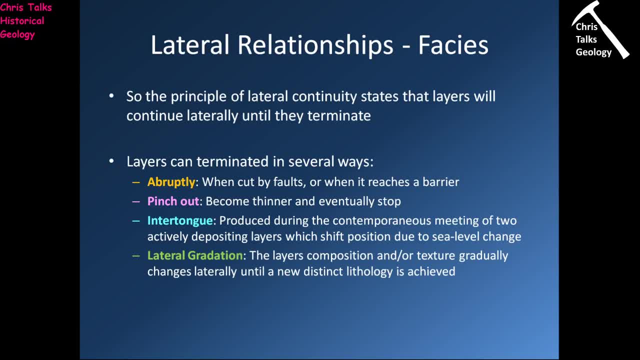 environment, and we can see that because the rocks change. So the question then is: well, how do how did the transitions between these fasces actually occur? Well, the transitions can occur in one of four ways. First of all, they can- it can be an abrupt transition, So you can simply have 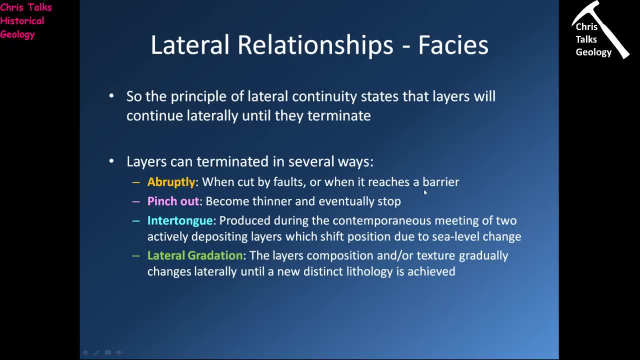 your rock is cut by a fault, so, or just some kind of barrier, So your layer of sediment will just simply just, you know, butt up against something and it can't go any further. So a classic example of that would be something like a river, So in your river channel, where the river is actually. 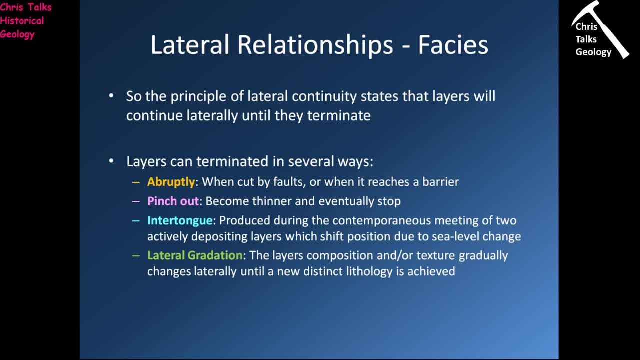 contained. you obviously have your sequence of river sediments, your channel sediments. Then, as soon as you step out of the river, those channels, well, those channel sediments, are stuck in the river channel, aren't they? They can't get out. So as soon as you step out from the river, 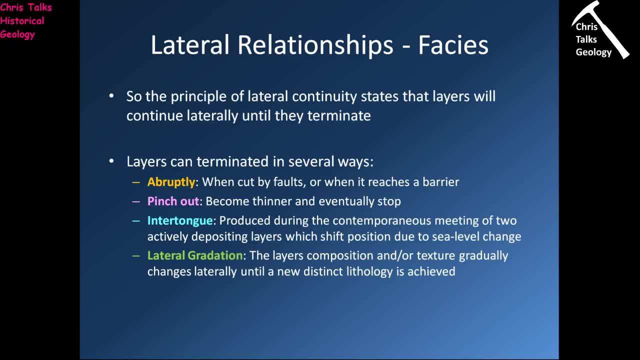 channel, you're in an environment of the flood, you know in the floodplain environment. So now you're, you know you're out of the water and you're into a dry environment. So in that case we have an abrupt transition: The edge of the river channel, the river sediments. 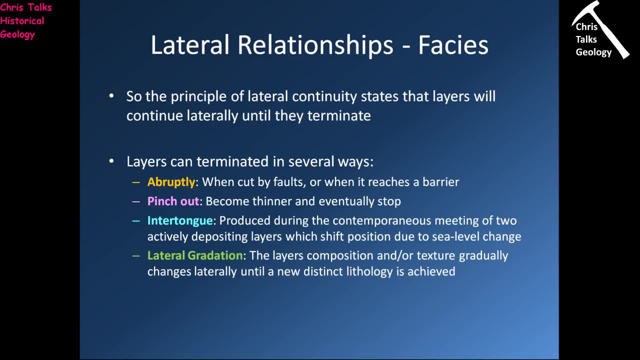 stop at the edge of it and then you transition into a new environment. Another thing that can happen is your layer of sediment can steadily get thinner and pinch out. So obviously, the further you go from the sediment source, the less material there's going to be, and so your layer of sediment. 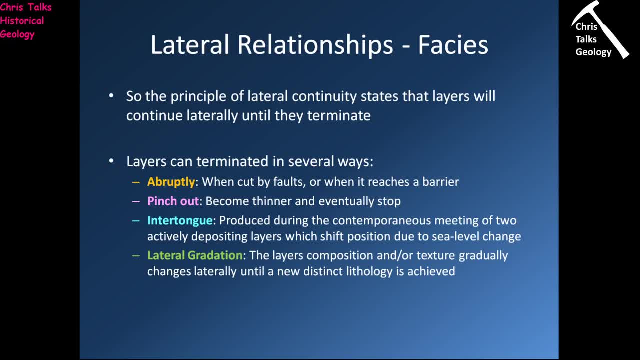 is going to steadily get thinner and thinner and thinner and eventually that layer will simply pinch out, disappear and a new layer of sediment will take its place. Now we also have something which is called intertonguing, and this is where we have multiple layers of rocks and they produce a distinct zigzag pattern, and it's the result of sea level change. Now I'm not going to worry about it too much because in a few slides time I have some reasonable diagrams which hopefully will show you what's going on in a reasonable level of detail. 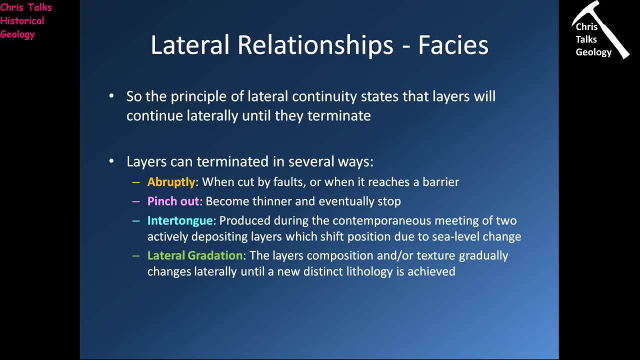 A far better level than I could possibly explain it. And finally, we have lateral rotation, Radial gradation, And that's when your layer of sediment slowly grades into a new sediment. So our medium energy beach sediment, which is very, very sandy, might steadily become more. 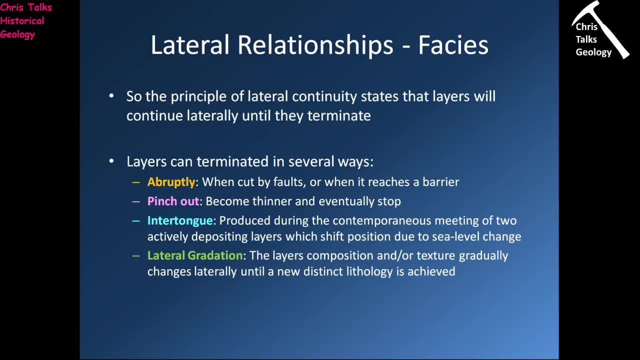 and more and more mud rich as we move from medium energy to low energy. So as you move from the medium to the low energy environment, the amount of sand decreases and the amount of mud increases And you have this gradational change going from the sandy beach sediments. 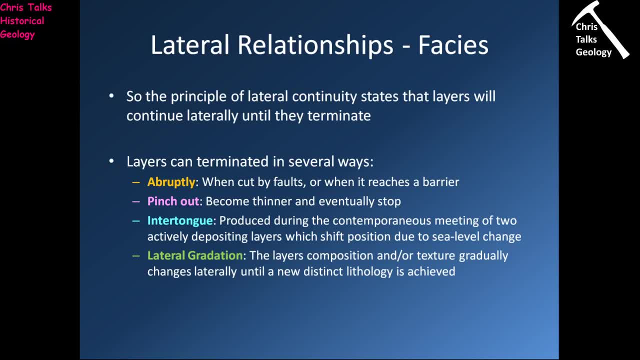 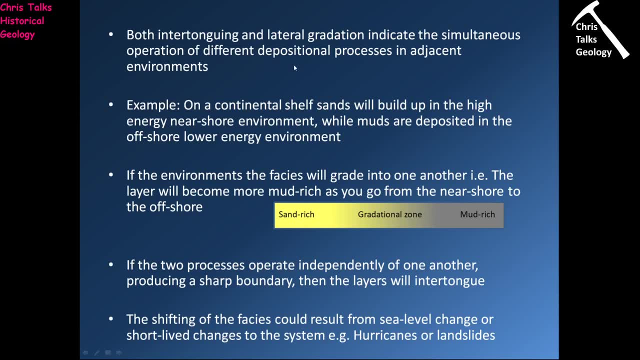 to the muddy, low energy sediments. So both intertonguing and lateral gradation indicate the simultaneous operation of different depositional processes in adjacent environments. So in both these instances what we have is we have two different depositional environments right next to each other at the same time. 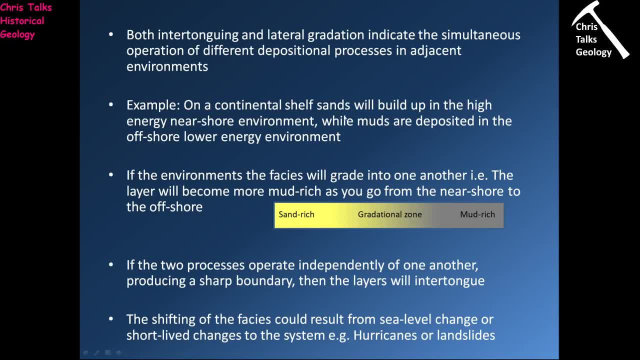 So a good example is the one we've been discussing: the continental shelf. you'll have a sandy pode environment closer to the coast, which is the, the beautiful beach of s bloat, the continental shelf. you'll have a sandy environment closer to the coast, which is the the muddy coast, which is the the muddy beach. 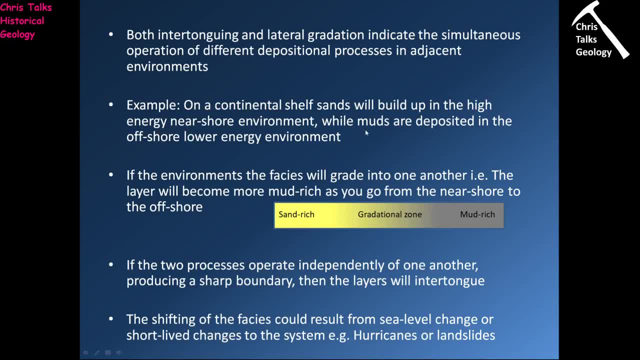 coast, which is the the higher energy near shore environment, whereas you'll also have, whereas you'd have, muds deposited further out to sea in a much lower energy environment. and so, if the environment is so, if the environment fascies will grade into one another the layer. 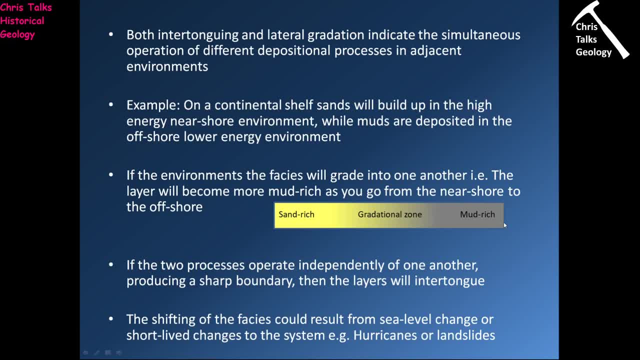 will become more mud rich. so if we- you know, this is very simplistic diagram is just trying to show that process. so here we have our moderate to high energy beach environment, which is sand dominated, and here we have our low energy mud rich environment. well, in the case of a gradational 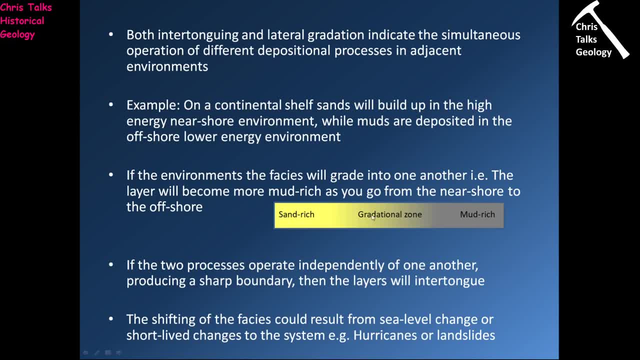 boundary. you're going to see, the amount of sand will steadily decrease as we move this way and the amount of mud will steadily increase. so if the processes in these two environments operate independently of one another, however, you're going to get a sharp boundary. so in this case, the two environments are operating. 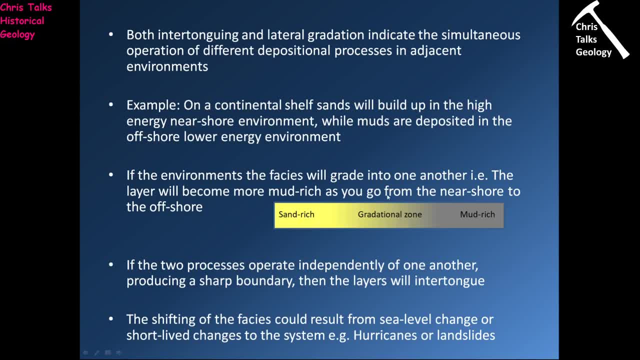 kind of together. there's this gradational zone between the two, where both environments overlap, so there will be some instances, though, where these two environments will operate completely independently of each other, and that's going to produce a sharp boundary, so it's going to be sand rich, boundary, mud rich, okay, and in that instance, we're going to see indications of things like 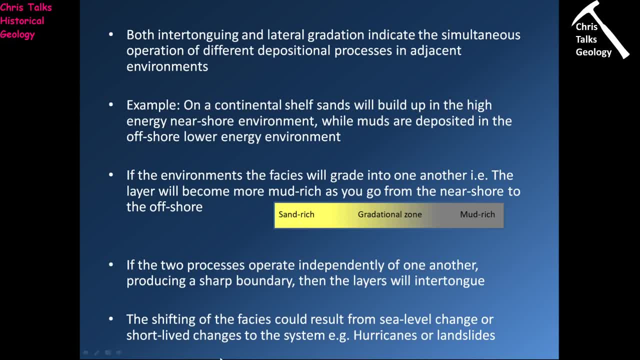 intertonguing in our sedimentary sequence. and this intertonguing, this zigzag, as i said, is the result typically of sea level change, or it can also be the result of short-lived changes, so things like hurricanes or landslides causing the the positions of the boundaries to shift slightly over short. 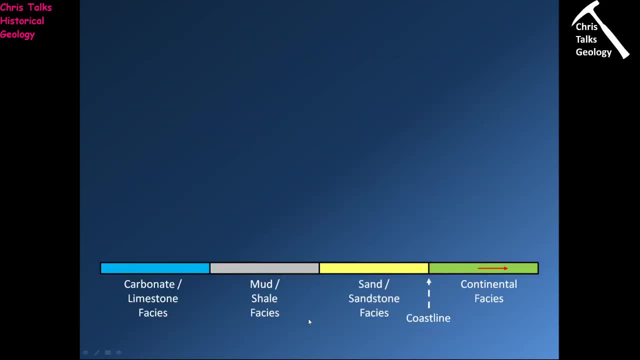 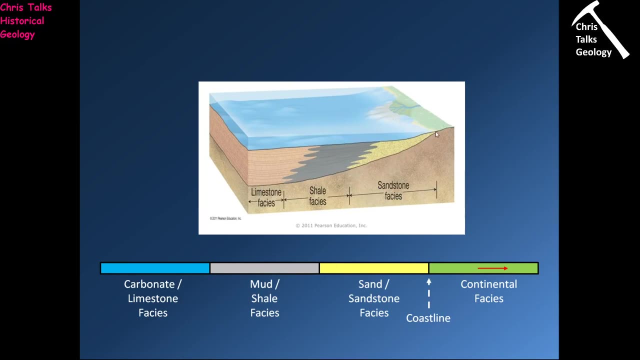 periods of time. so here's our situation, so this is what we've been talking about. here's our continent, here's our coastline, and we can see as we move into deeper water, we go from a sand-dominated environment, because this is a moderate energy environment. we then transition into a low energy, mud-dominated environment, and then we step out into a 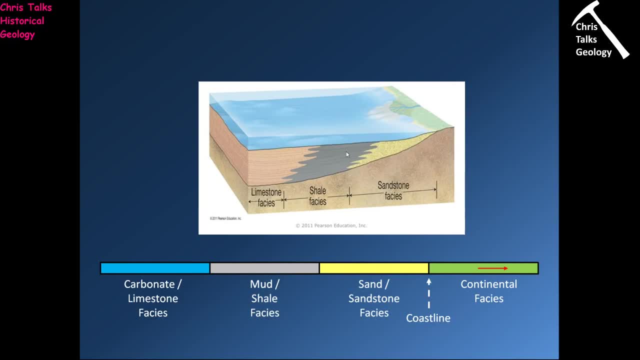 carbonate-dominated environment. so this is the classic set of rocks we expect to see on a continental shelf: sandy closer to the coast, as we go into deeper water, they transition into muddy and then finally, the mud will give way and it will be replaced by carbonates. and so if we would 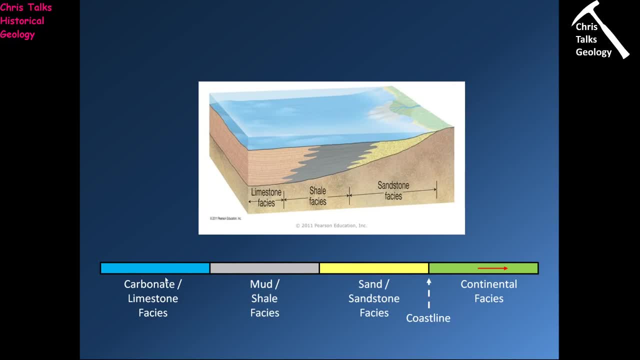 just take a slice through this. what we would see is we'd have a sequence that goes: carbonate or limestone fasces, mud fasces, sand fasces and then continental fasces, the land itself. okay, so if we just moved across here, that represents that. this represents this. 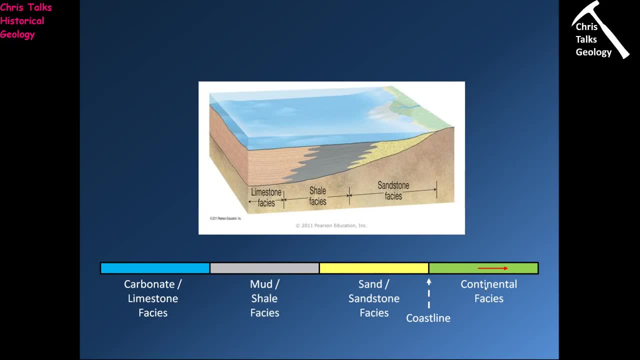 the net there represents this, and this bit is represented by the continental fasces. so what i'm going to do is i'm going to change the sea level, so i'm going to push the sea onto the land. so now, all of a sudden, your land is going to be covered by a moderate to high 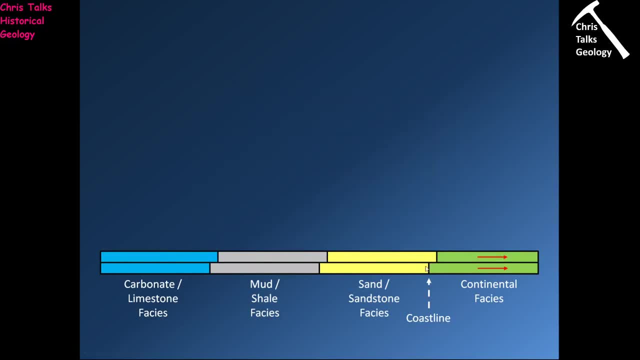 energy, beach environment. so our continental fasces are going to start to be covered over by the sand fasces. at the same time as the sand fascia starts moving inland, the mud and carbonate fascia is going to follow it, and so we're going to see the mud fasces superimposing themselves. 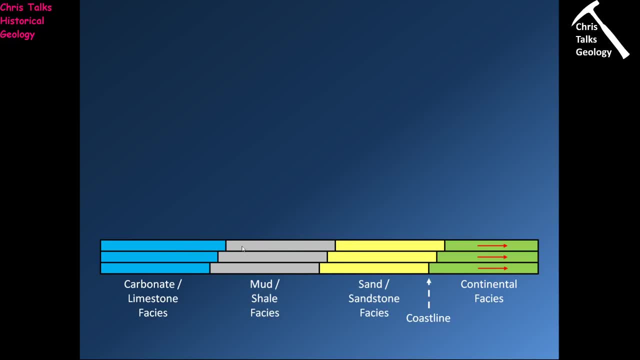 over the top of the sand fasces and the carbonate fasces over the top of the mud fasces. okay, and we can see that, as the water's moving inland, we have these fascias are moving over the top of each other. then there's going to be a marine regression, the sea is going to start coming off the land and 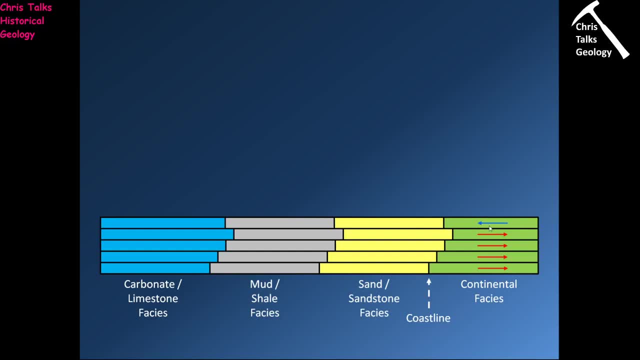 go back into the ocean. well, in that case, all of a sudden, your land, which was covered by water, is now exposed again. so now it's a continental environment. so we're going to see the fasces change. we're going to get different rocks forming. obviously, as the sand fasces moves back into deeper water, the mud fasces will also. 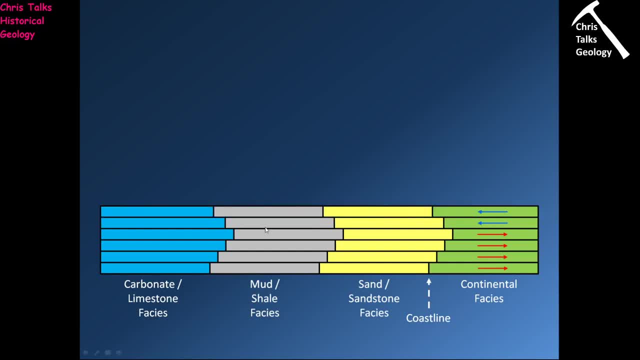 move back into deep water, and so will the carbonate fasces, and so we'll see the fasces move away. then there'll be a change in sea level again. we'll see the fact, we'll see the sea level moving in, and then we'll have the the fasces begin to move inland. so in that, once again we have the sand. 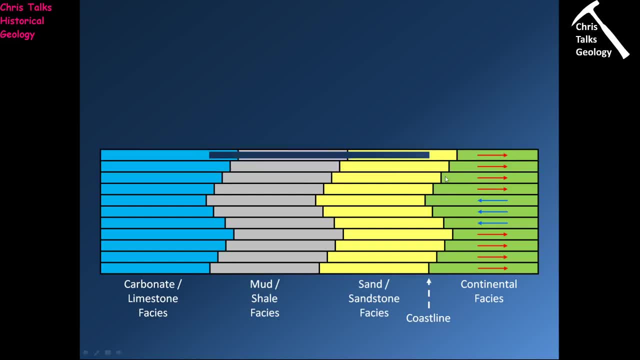 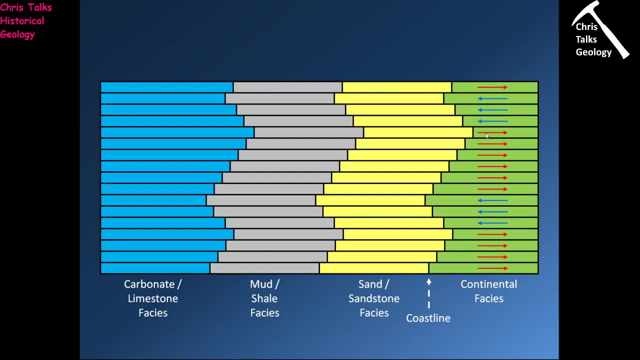 fasces moving over the top of the continental fasces, and you can see this happening. so we've got it moving on land. then we have a reversal and then we have another marine transgression, and so what you can see here is there's that zigzag pattern, that intertonguing that we were 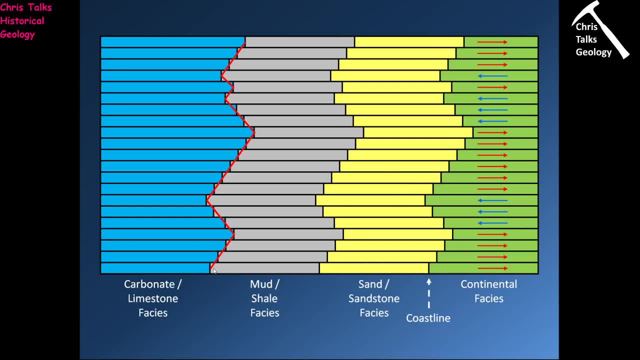 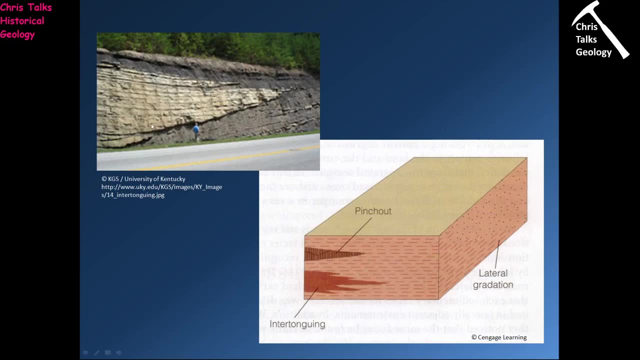 talking about. so, as the sea level changes, it causes these fasces to shift position. they'll superimpose themselves over the top of each other and it leaves this very, very distinct zigzag pattern. when you look at the fasces vertically- and so i appreciate- it's an absolutely terrible picture. 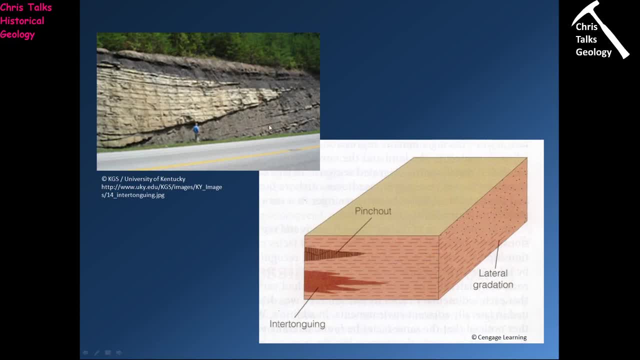 but you can see that going on here. so over here we have a mud fasces in this kind of grey brown and here we have a sand dominated fasces in this kind of yellow, white and you can see we have these zigzags. so it comes out here steps back, comes out a long way. 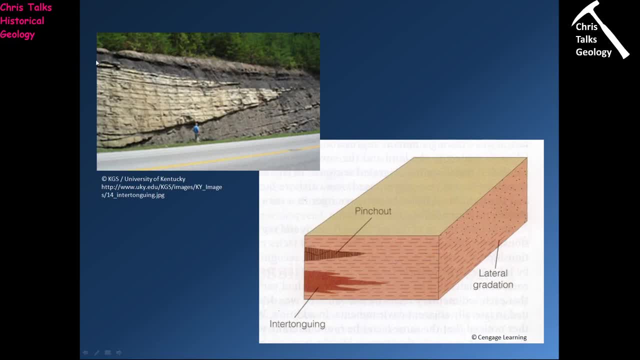 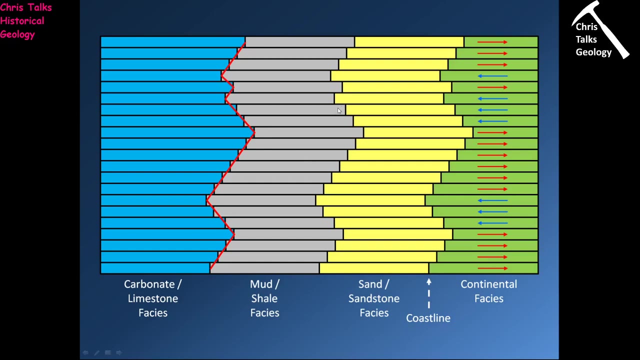 steps back, comes out again, steps back, And this is a fasci superimposing itself over another. So in this case we have sand fasci superimposing itself over the top of the mud fasci. So if we just go back, we have a sand fasci superimposing itself over the top of a mud fasci. 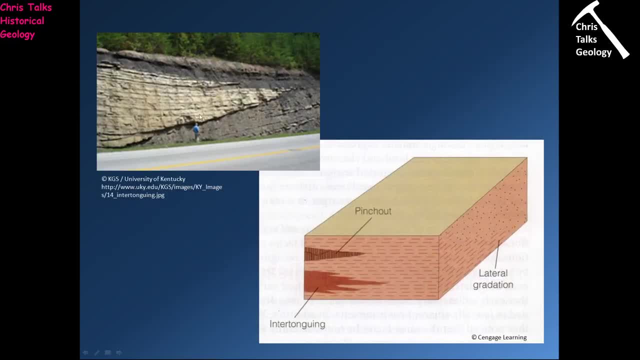 So this is probably going to be produced by a marine regression And this diagram here kind of just summarizes the differences. So obviously, when we have lateral gradation, we change from one sediment to another gradually. In the case of intertonguing we have distinct fasci which have sharp boundaries, hence the sharp contact.